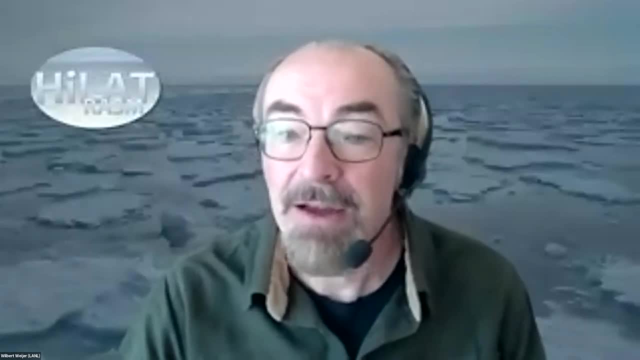 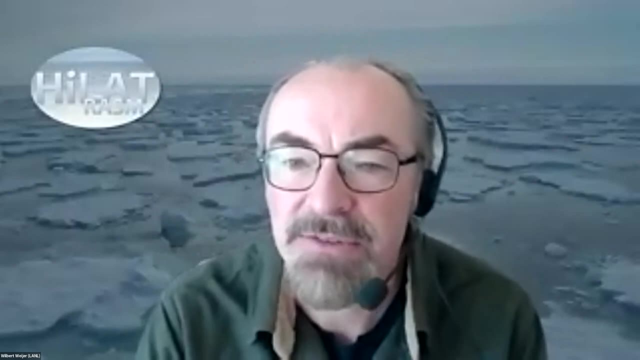 Influence from the Arctic, from the Atlantic and the Pacific, with important impacts on the regional atmosphere, sea ice and ecosystems, While, on the other end, the water mass transformation processes in the Arctic produce water masses that affect and contribute to the global overturning circulation. 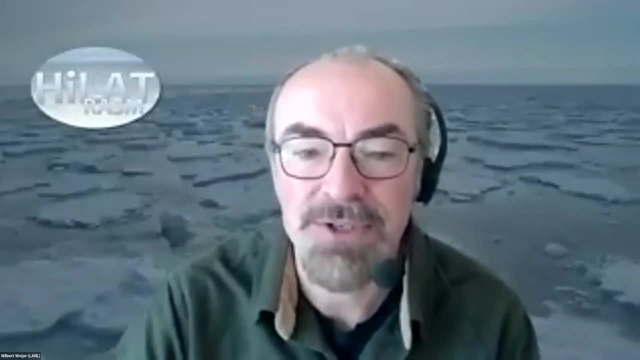 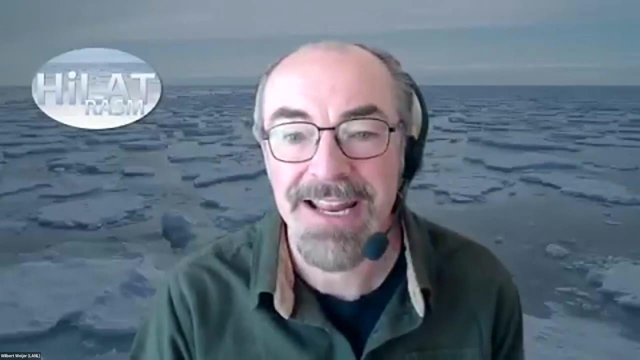 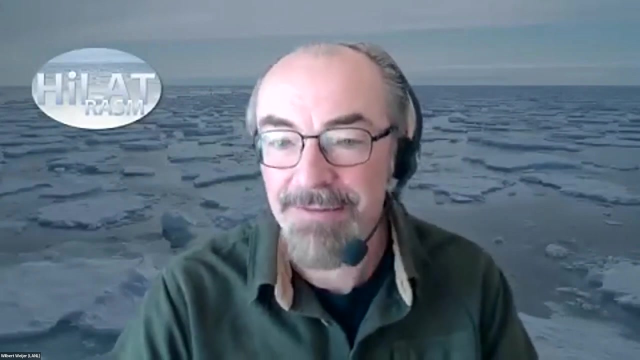 And understanding these two-way interactions is critical for our ability to project the evolution of the Arctic Earth system in general. But today we will have two presentations by very distinguished scientists. The first speaker will be Igor Polyakov from the University of Alaska, Fairbanks, who is also affiliated with the International Arctic Research Center. 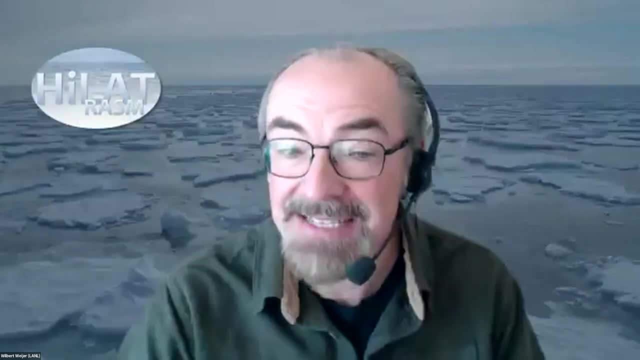 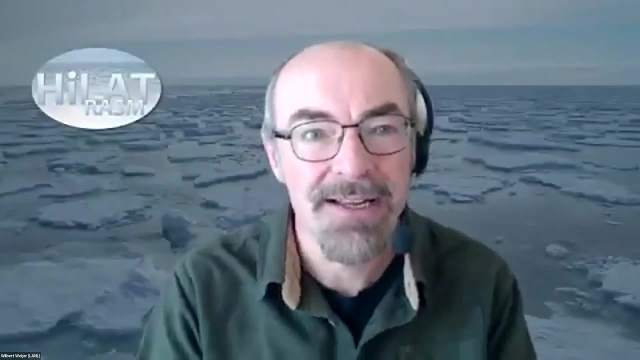 And he will talk about the status and trends of the Arctic Ocean circulation. So the presentation should not only be 15 minutes, with some time for questions afterwards and hopefully at the end of the presentations we will have some time for some general discussion. So we'll start with Igor. 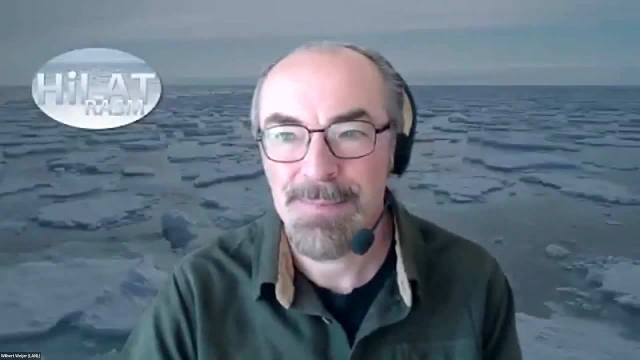 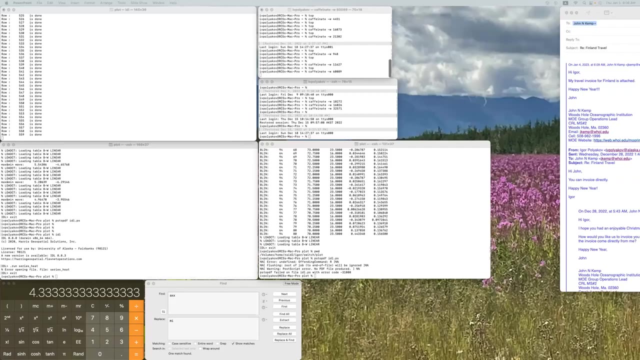 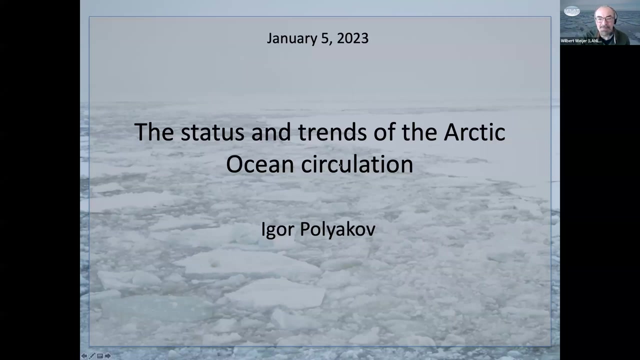 And with that I'll hand it over to Igor. Thank you very much. Please remember to mute yourself if you're not speaking. Do you see my presentation? Yes, we do. Okay, good Looks great thanks. Happy New Year and thank you very much for inviting me to give this talk. 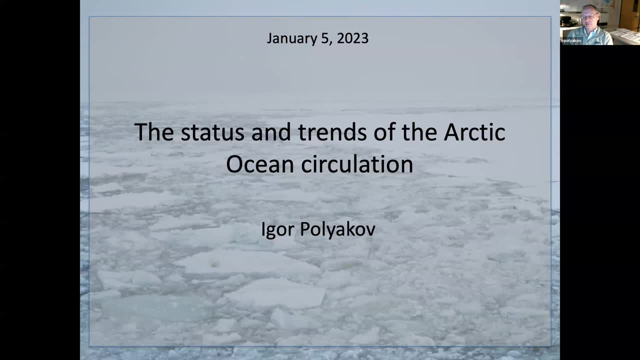 It's very limited in time So it will be very sketchy, very brief, But I hope I will deliver a message about these big changes we currently observe in the Arctic Ocean, And my focus will be on Arctic Ocean circulation. First I will touch pan-Arctic changes. 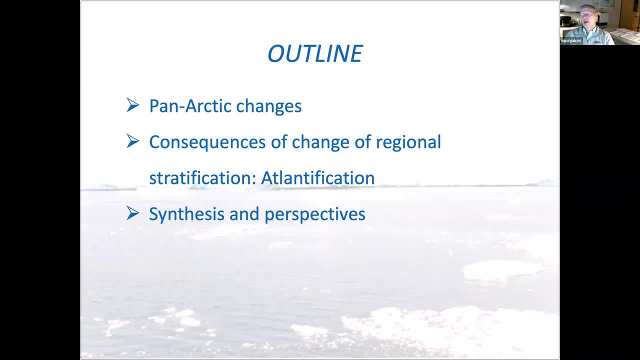 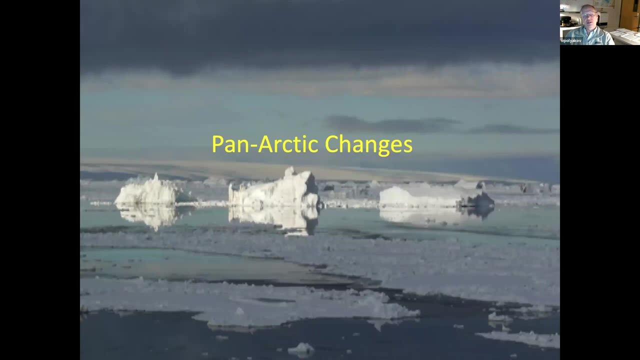 That will be sort of an introductory note, And then I will talk about consequences of changes of regional stratification And I will talk about Atlantification. I will finish my presentation with some Synthesis and Perspectives, And so let's talk a little bit about pan-Arctic changes. 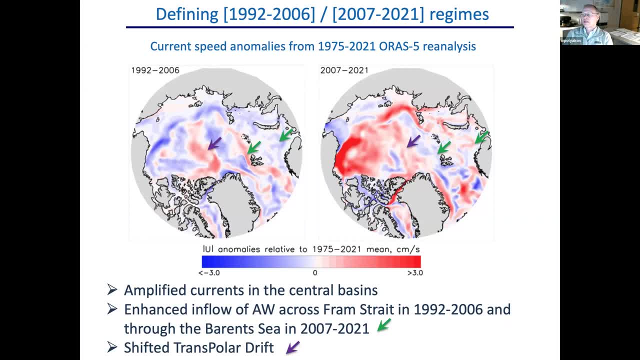 For this plot I used the reanalysis data, And this reanalysis- ORAS-5, proves to me to be extremely helpful. extremely useful to deliver a lot of useful information about Arctic Ocean circulation and its changes. So here, in these two plots, you see anomalies. 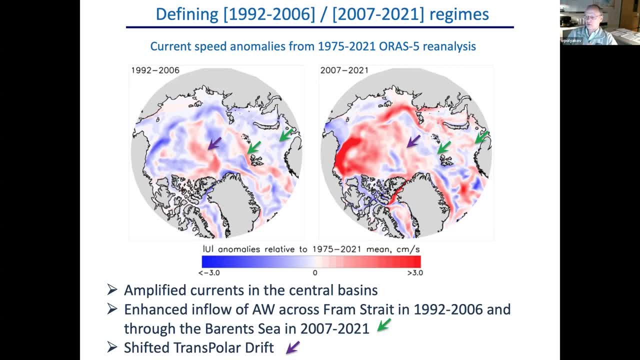 So here in these two plots you see anomalies. So here in these two plots you see anomalies. So this of current speed, Anomalies relative to mean 1975-2021.. And I would like to stress big differences between the state of Arctic Ocean circulation based on this reanalysis. First of all, you see that the 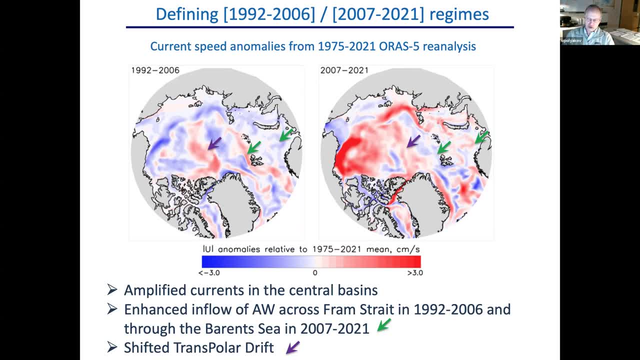 recent 15 years are associated with very strong increase of oceanic currents in the Central Arctic. That is shown by dominating red color. This is true for amplified Beaufort gyre- here an anti-cycloning Beaufort gyre. This is also true with amplified currents in the Eastern Eurasian. 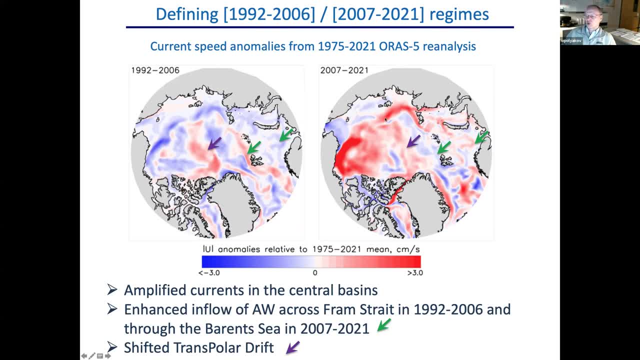 Basin along the slope. This is also associated with change of the position of transpolar drift, which was closer to the Lomonosov Ridge in the recent 15 years compared with the previous 15 years. You see this as indicated by this purple arrow. You also see a very interesting feature. 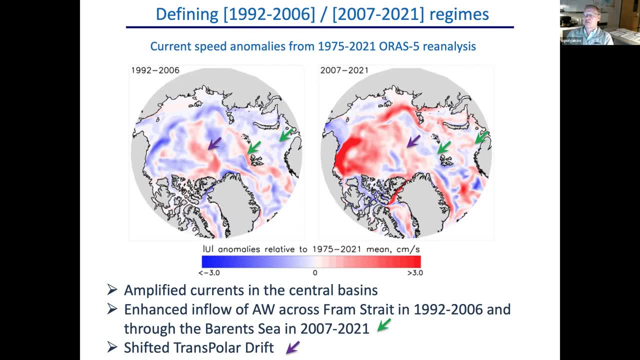 of shift of the different impact of influx through Fram Strait and the Barents Sea. In 1992-2006, the dominant inflow was through Fram Strait, as indicated by this red branch of influx through Fram Strait, whereas in the last 15 years the dominant branch was the Barents Sea branch. 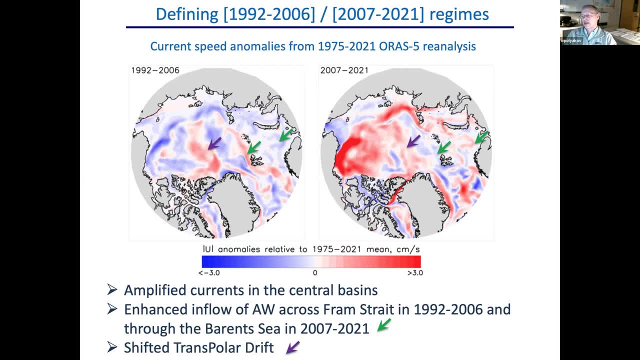 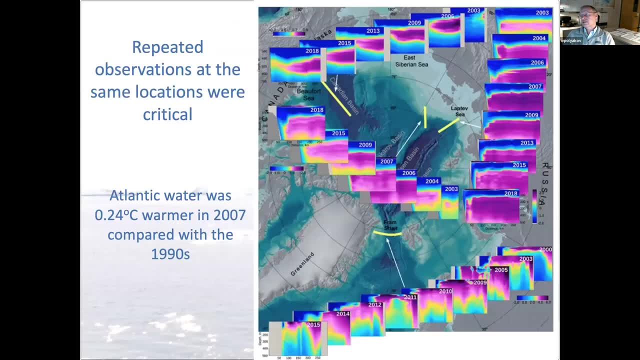 These are very important, very interesting findings and I would like to emphasize them because they are important for the future discussion. Next slide shows repeated cross-sections made along the certain lines. For example, this cascade of cross-sections of water temperatures are associated with annual 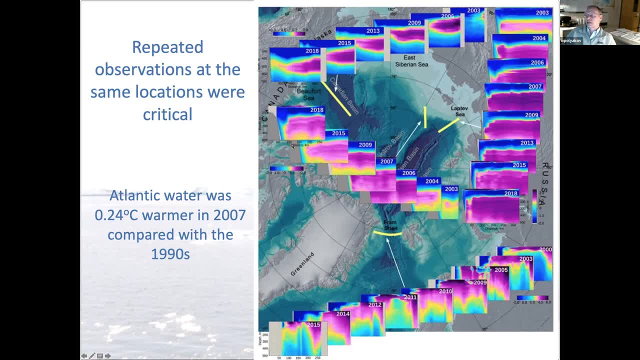 observations along this line in the Eurasian Basin and in the filosofy. I show four positions for this. these repeated cross sections: Each cross section here shows water temperature. So red color indicates very warm water, blue color indicates very cold water. 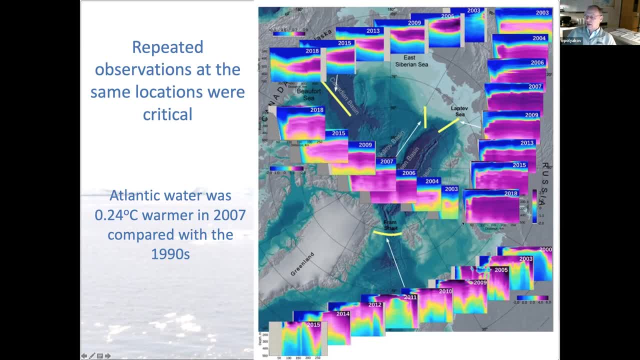 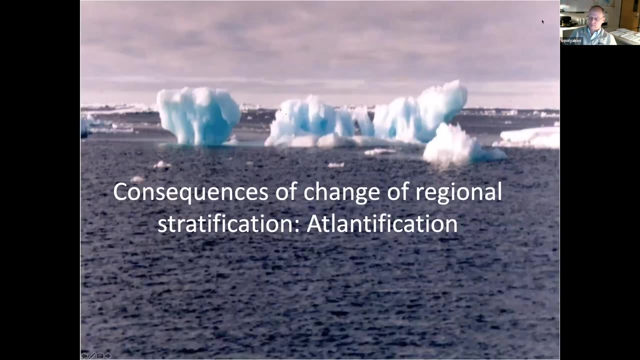 and this is vertical axis depth. This is a horizontal distance from the slope And you see this cascade of water temperature. cross sections show a dramatic increase of water temperature in the interior from 2002,, 2003, through 2007,. eight nine. 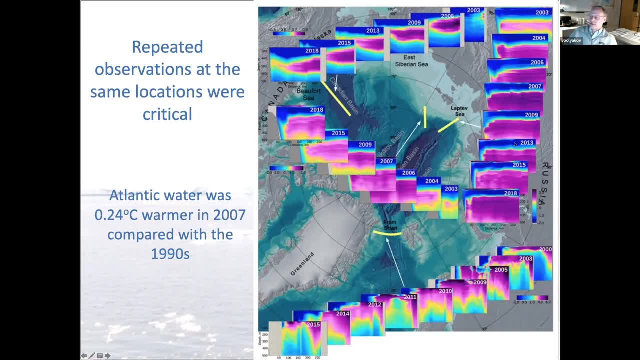 where the temperature was at peak, And now you see the slight decay of water temperature compared to the peak one, but still the water in the ocean interior is much warmer compared to the beginning of 2000s. What is also important to emphasize is that at the top of this cross section, 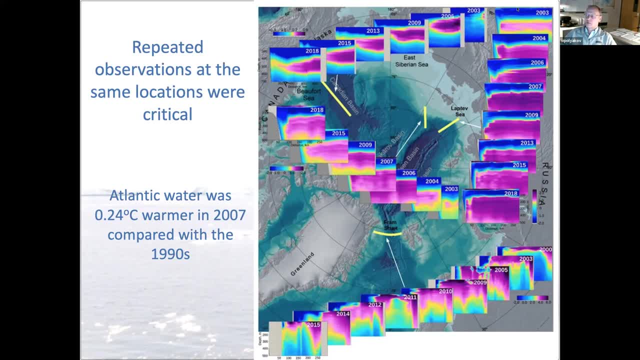 so we see impact or real impact of surface warming. There was nothing like that in the early years because, according to our observations, this area was completely ice covered. So that's a big transformation in the Arctic Ocean when the seasonal ice zone moved from the shelf into the deep ocean. 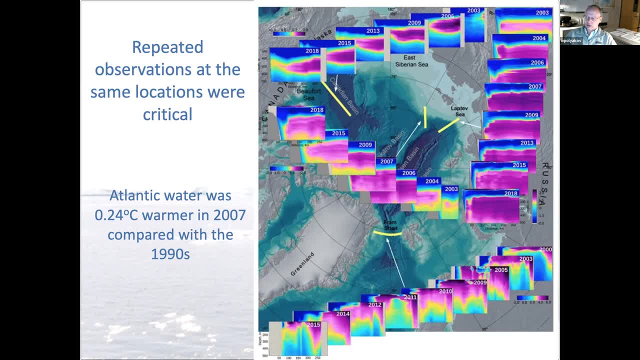 It's very important to emphasize that, together with the change in the water-heat-content in the ocean interior, there was a change in the surface in the Halleck line. In this plot, Halleck line is indicated by this warm. 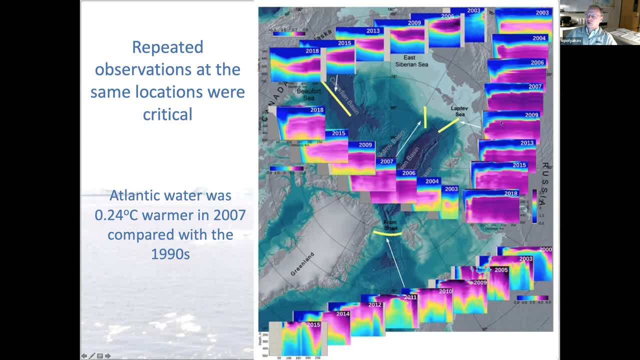 or this cold layer where the temperature rapidly goes from high values to very low values at the surface. Salinity in this layer also decreases rapidly And this layer was very important. Halleck line was very important in the past, serving as a very strong barrier for the oceanic heat. 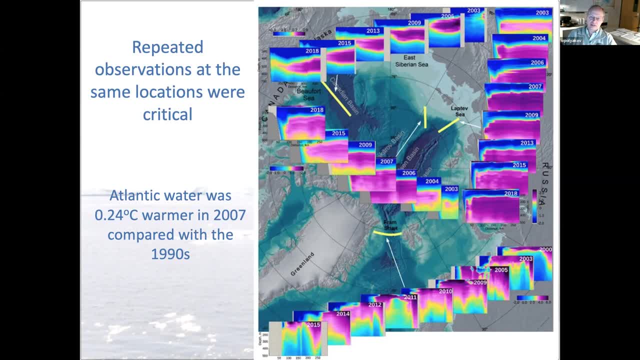 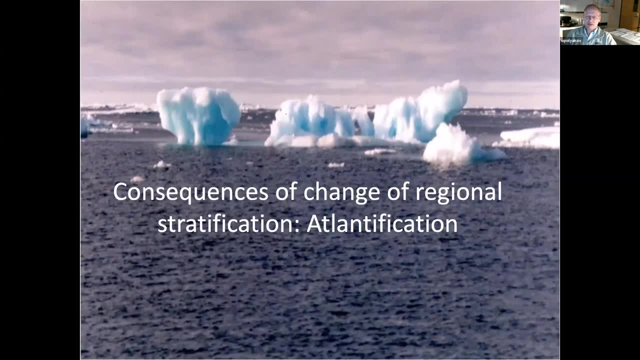 to penetrate through the Halleck line and reach the bottom of sea ice and having impact on sea ice formation. So that will be basically the story of my major part of the presentation where I will discuss consequences of changes of original stratification in the Halleck line. 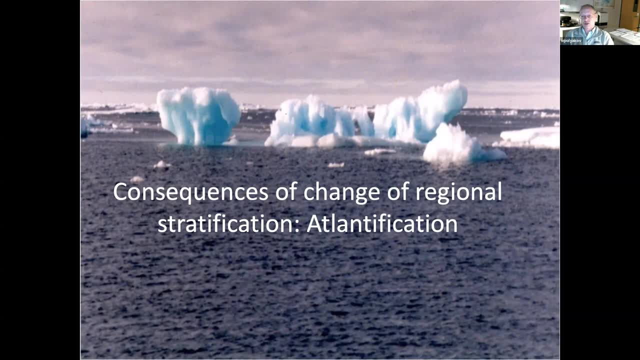 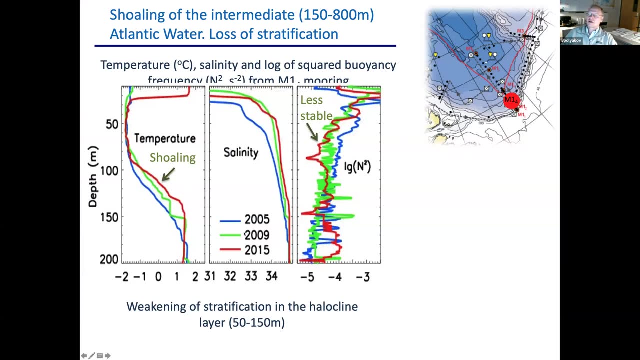 and associated process, which I call Atlantification. These changes in the Halleck line are clearly seen in this plot of vertical profiles of temperature, salinity and buoyancy frequency. These measurements are made at this spot, which is climatological spot. 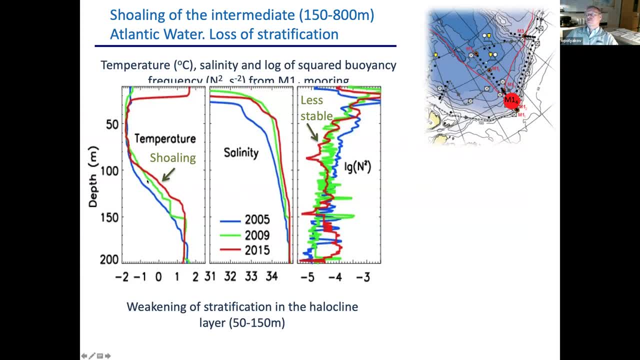 of our observational program NEBAS, And from these profiles of temperature you see shoaling of the Atlantic water. Shoaling means that in time the boundary of the Atlantic water becomes closer and closer and closer to the surface, making Atlantic water heat. 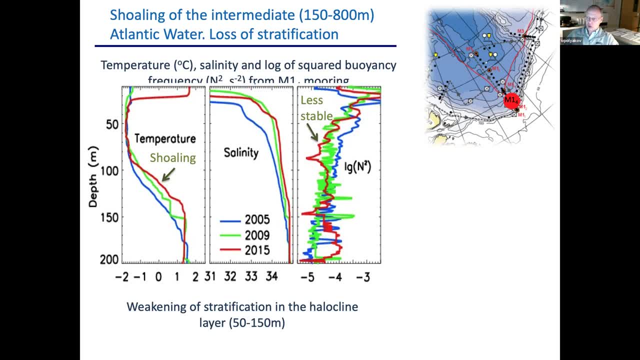 more available for mixing from the surface. But most important for my discussion today is that at the same time Halleck line became weaker, weaker, weaker and weaker. Stratification in the Halleck line was much less in recent years compared with the past. 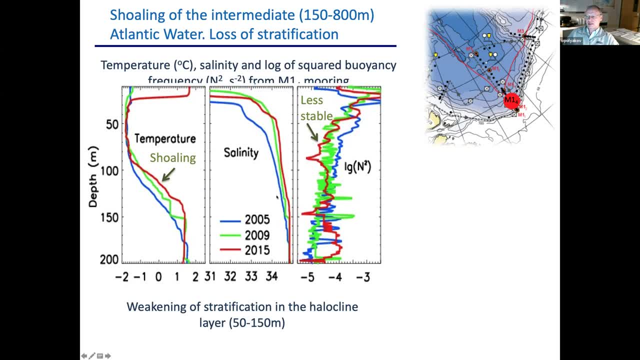 And this is clearly identified by these profiles of salinity, which define the profiles of density. you see that in time, the profiles of salinity becomes closer and closer to vertical. That means that the vertical gradient of density becomes weaker and weaker, making the Halleck line, this barrier, weaker and weaker. 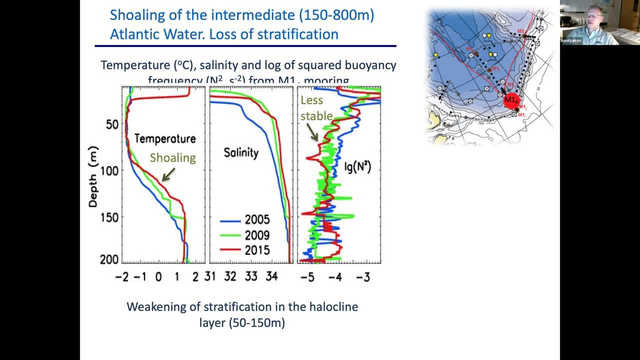 for mixing and propagation of heat from the ocean interior to the bottom of sea ice. Weakening of the Halleck line was identified as a process which is influenced by influx of denser water from the Barents Sea. That's why I call this process Atlantification. 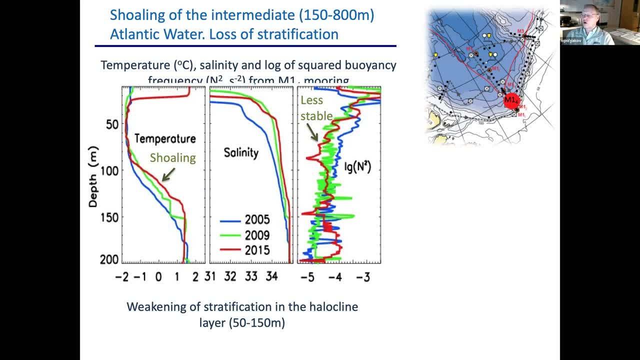 We definitely see impact of advection of anomalous features from sub-Arctic seas into the Arctic And, together with local changes, climatological changes. this remote induced changes play a very important role in shaping the current state of Arctic ocean sea ice and atmosphere. 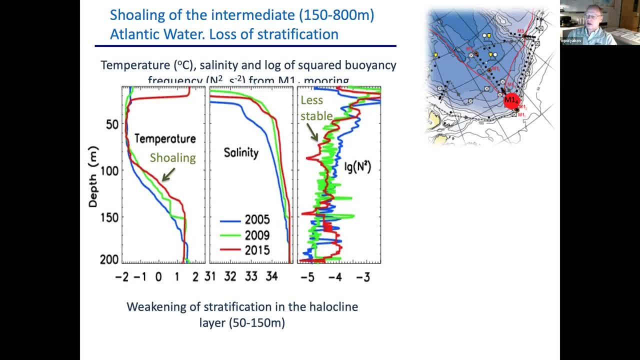 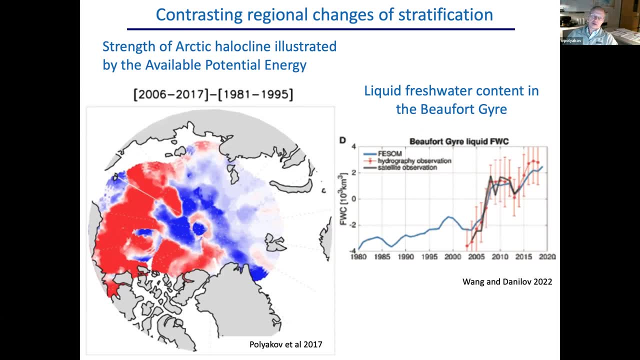 You may say these are just three profiles from one spot and maybe the Arctic ocean was not changed considering its stratification, but this is not true. We made an analysis using historical observations from ships, ITPs, from all possible sources of information. 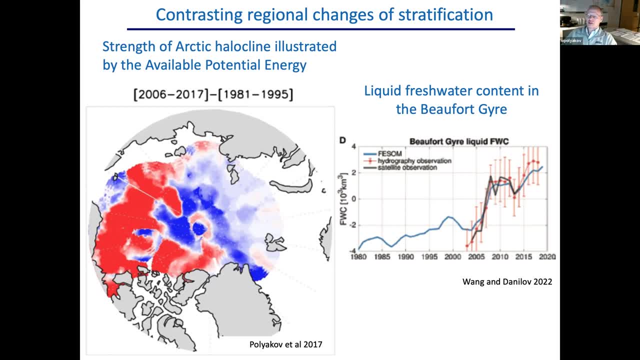 and build this picture of available potential energy. This particular plot shows compares available potential energy for the recent years, 2006,, 2017, versus what was observed more than a decade above. So these are anomalous picture of available potential energy. 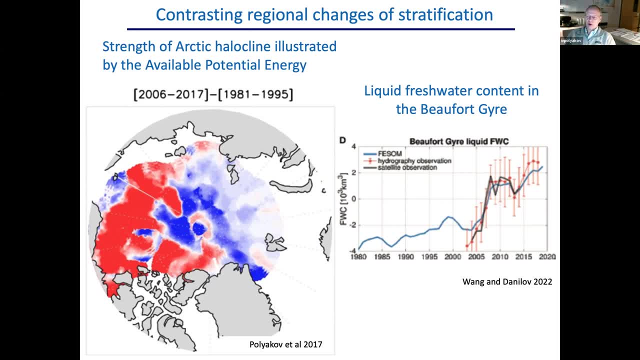 And available potential energy is calculated for the upper ocean, including surface mix layer and Halleck line for this plot, In physical interpretation of this plot, is like that: Available potential energy. the level of available potential energy characterizes the ability of water to be mixed. 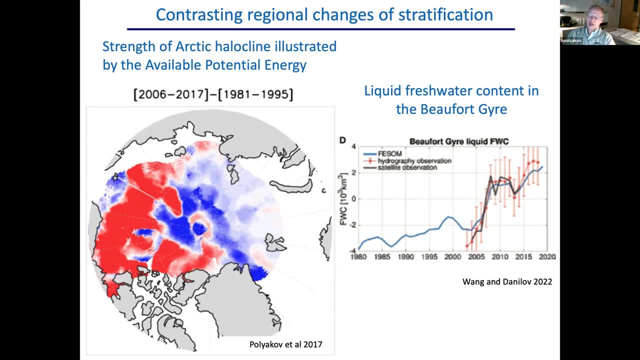 Less energy means more ability of layers to be mixed, whereas increase of available potential energy identifies the case when it's much more difficult to mix water. So you see that the process of accumulation of fresh water in the Canadian basin was associated with increase of available potential energy. 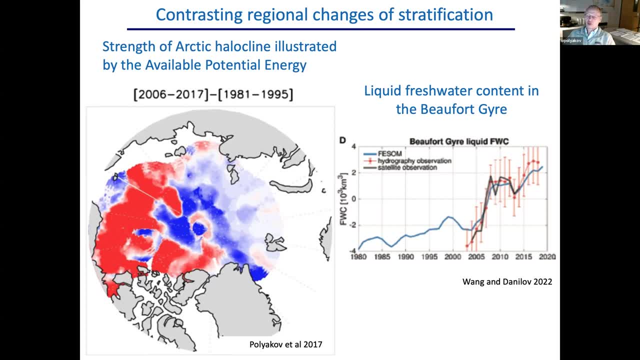 That means that the Canadian basin is now more difficult to mix compared with Eurasian basin, which was losing available potential energy. become more accessible to mixing- And this plot here confirms this argument- that the Canadian basin became much more stratified in recent years compared with the past. 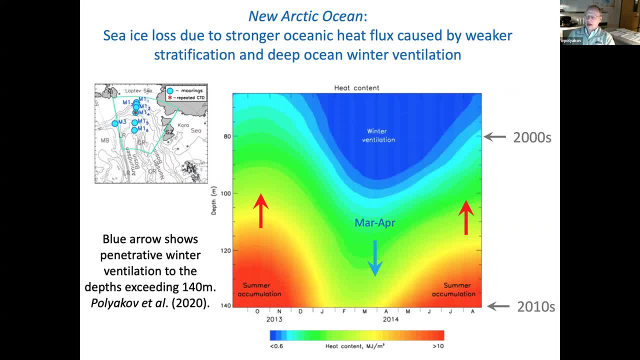 This Changes in the Eurasian basin had dramatic consequences for the mixing. This is a segment- one year segment- of a mooring record from many records we have. This map shows location of moorings where we have similar records and they basically show similar situation. 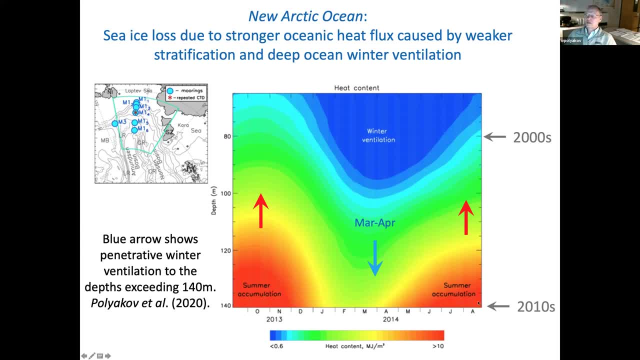 And this plot. this panel shows the heat content within the upper 140 meters Heat content within the upper 140 meters. Heat content may be also interpreted as the mean temperature And it's smooth to keep seasonal cycles for easy interpretation. So you see that at the beginning of the year 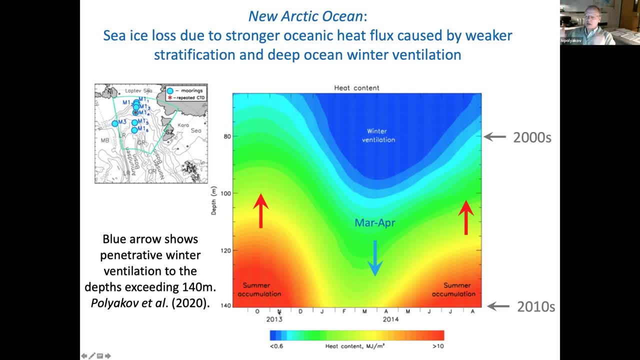 the system accumulates heat and this heat goes from the bottom of this panel, from the ocean interior- This is Atlantic water heat- And without mixing from the surface, this heat is accumulated in the upper layer. When winter comes, sea ice formation occurs. 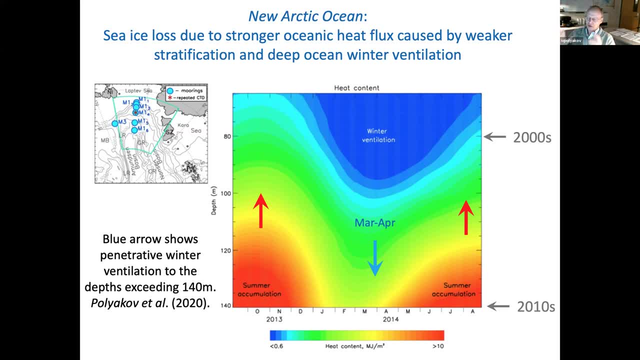 and this sea ice formation cools the water and salt release during sea. ice formation mixes the upper ocean And you see, during the winter there is a great deal of ventilation of the upper ocean. It's also important to emphasize that this mixing goes well beyond the surface mix layer. 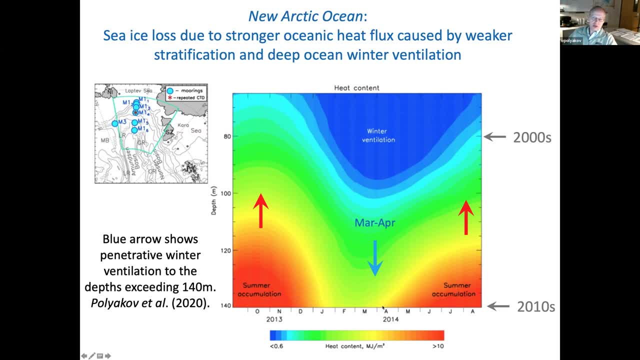 You see that I limited this plot by 140 meters, where the signal is statistically significant, but actually it goes to 160, 170 meters. This is already the Atlantic water by itself proper. So we definitely see that winter mixing gets a lot of heat from the ocean interior. 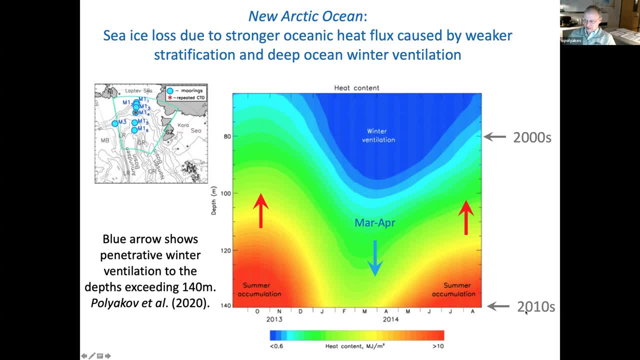 And this arrow here indicates the depth, statistically significant depth of sea ice formation. So we can see that there is a lot of surface ventilation, whereas just 10 years ago ventilation didn't go beyond 80 meters. This is fundamentally different state of the ocean. 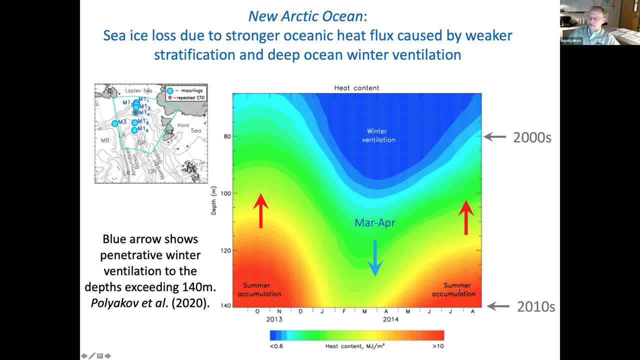 Then winter is gone and there is no ventilation from the surface and the system starts gaining heat again, And this cycle is repeated in time. Also, it's important to emphasize that by sea ice formation and cooling and salt rejection in the water, 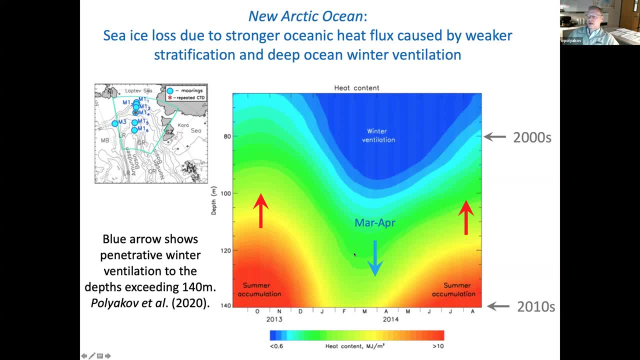 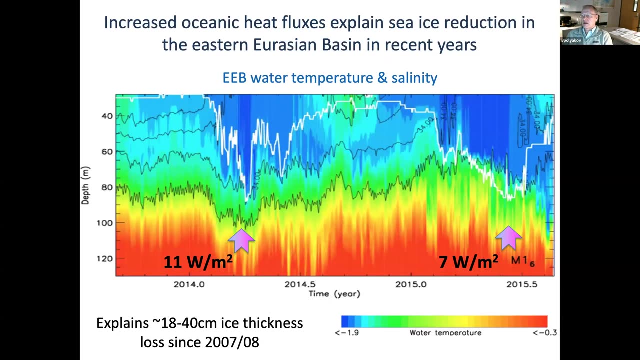 But you see that mixing goes well beyond the surface mix layer And this is already a different process, process of entrainment, where the internal waves play a critically important role in mixing of the ocean. Here is a record, raw data, So you can see the not smooth, not smooth. 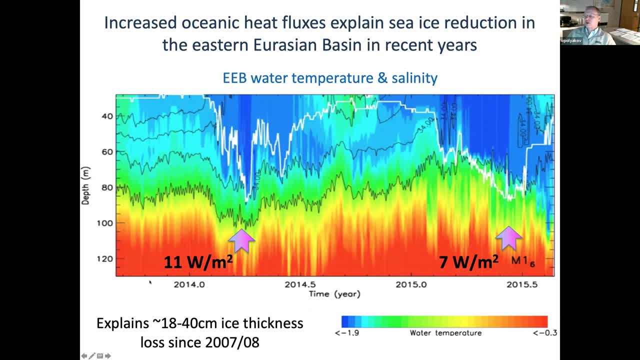 but raw data: temperature within a mooring record, And this plot shows two years of records. White line here indicates the depth of the surface mix layer And you can see that in winters the mixing goes to 80 meters, but the mixing associated with entrainment. 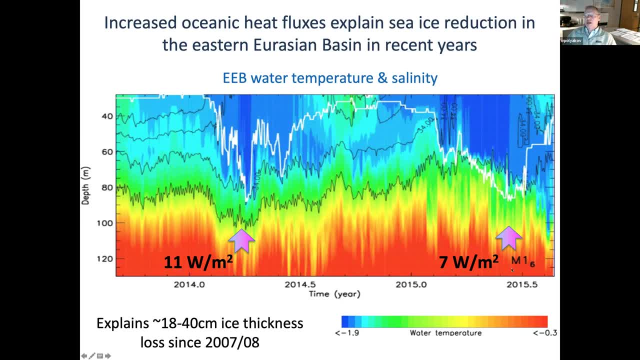 goes in much deeper layers. We can calculate the heat release due to this mixing in the system using these mooring records, just by comparing the rate of heat loss in winter, And by this approach we can estimate the amount of heat released to the bottom of sea ice or heat fluxes. 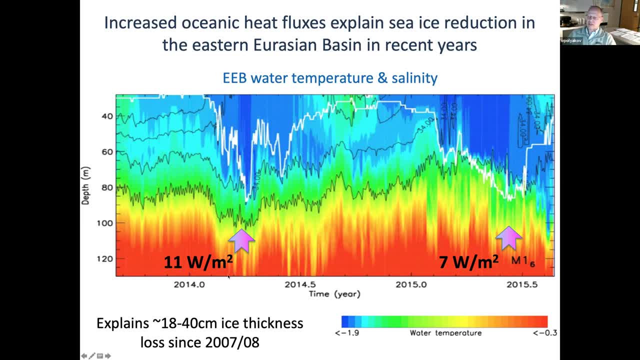 And doing this, we came to numbers of 7,, 11,, even more watts per square meter. We could compare these numbers with observations derived from previous years, 2007,, 8.. And we definitely see that this current heat flux due to weakening of stratification. 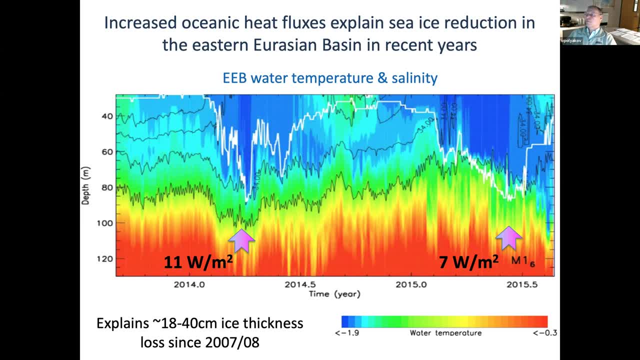 and release of Atlantic water heat to the bottom of sea ice, much amplified. This amplification of heat flux explains up to 1840 centimeters of additional sea ice loss due to this upward, additional, upward heat flux. This is a very big number. 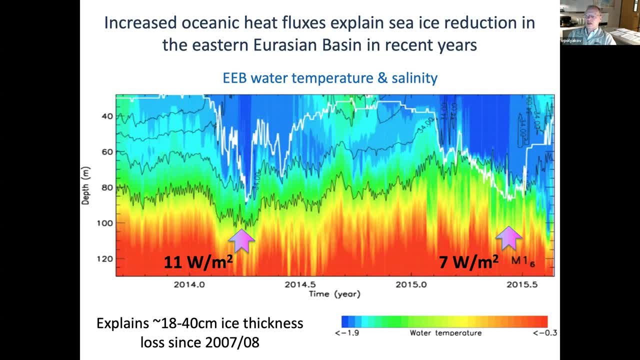 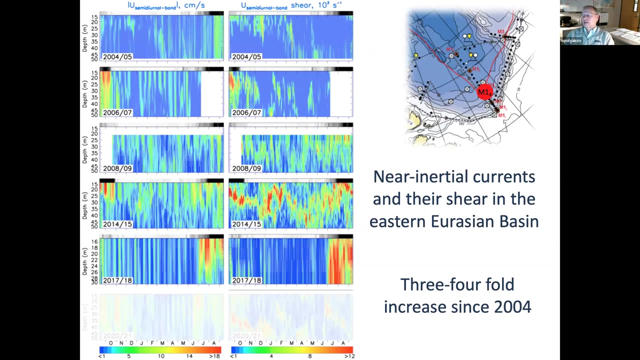 The ocean becomes critically important in shaping the state of sea ice in winter and producing different state of sea ice. before summer, sea ice melt in this area of the Arctic Ocean. This is not the only change in the system. We definitely see that all components of the system 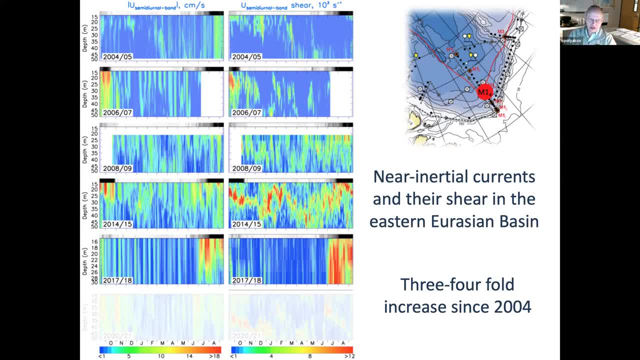 in Eurasian basin are changed Dramatically. So these are the records of ocean currents within the semi-diurnal band. This is depth, This is time, And for each panel shows one year record from our mooring. Its position is indicated here by this red dot. 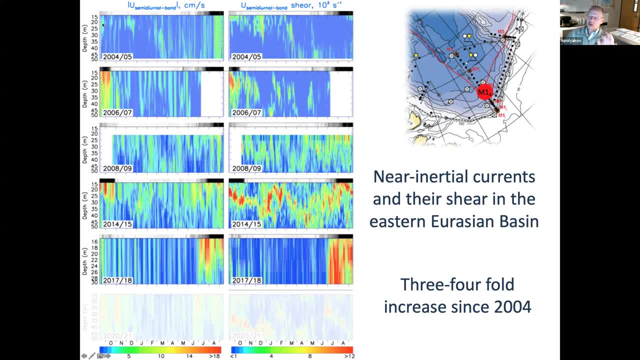 And you see that, within this very important band which incorporates tides and the sea, ice and the ocean, The current is very weak. It is very weak in 2004.. And then there is a very strong increase in current and inertial oscillations. 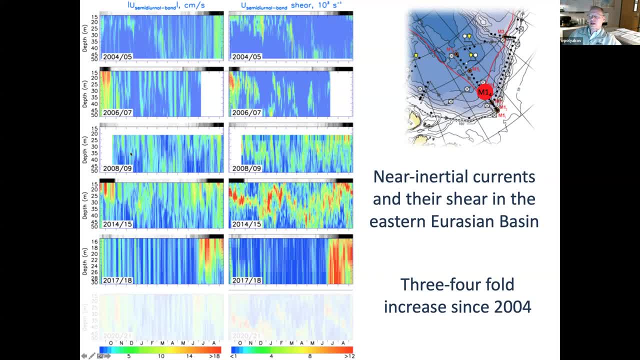 The currents in 2004,. five were pretty weak. The same is true for 2006, seven. Whereas in later years there was a great increase of the intensity of currents in semi-diurnal band, The other was an estimate of three, four fold increase since 2004.. 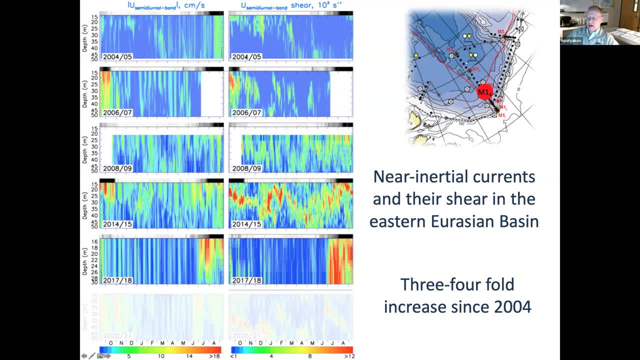 And at the same time there was a strong increase of vertical shear, of horizontal current. So this is a very significant change. horizontal currents: this shear is indicated in this column, so you see a lot of blue colors in early years meaning low shear, whereas there is a lot of shear in recent years and our collaboration 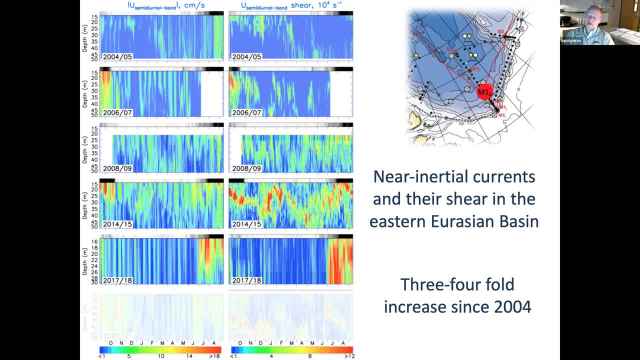 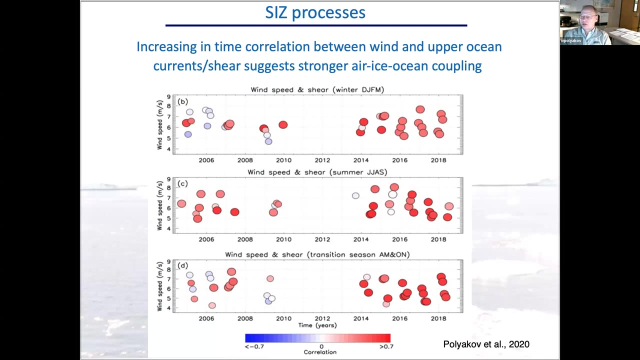 with modeling community told us, informed us, that this is basically due to very strong increase of berkley nictides. another process, very important process, is increase of coupling between ocean, sea, ice and atmosphere. because of all these changes, we expect to see an increase of coupling between these three components of the of the arctic climate system, and here are three panels. 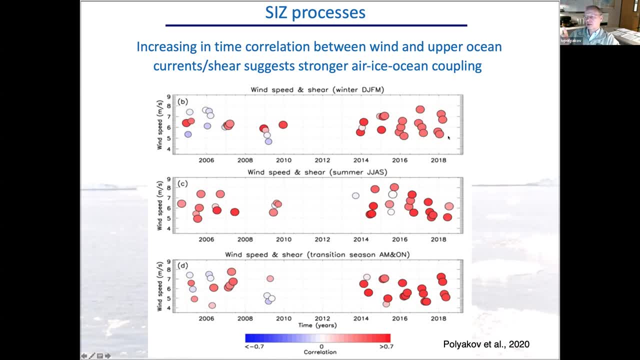 showing different things, but i would like to- you know, you know- concentrate your attention on the color which indicates the correlation between wind speed and vertical shear of horizontal currents, in winter upper panel, in summer middle panel and in transition period. so red color indicates strong correlation, blue color indicates much lower. 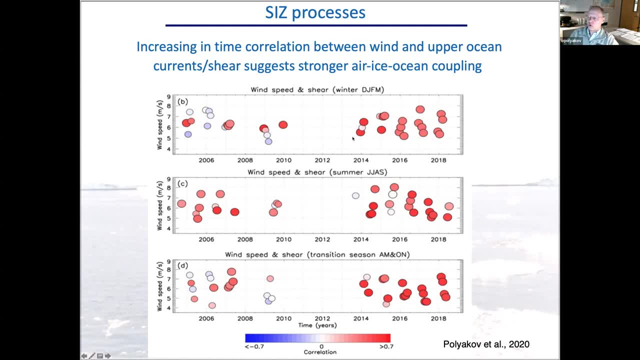 correlations, even negative correlation. so you see that for all seasons the correlation between wind speed and and shear- the same is true for currents in the upper 50 meters- is increasing in time, meaning that there is strong increase of coupling between atmosphere, ice and the ocean in eastern eurasian. 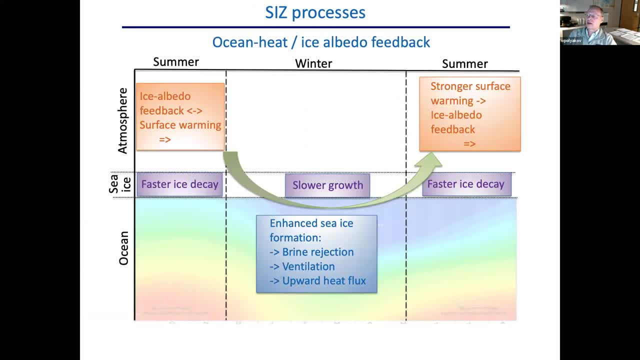 basin. based on these findings, we came to a idea of a feedback mechanism which is more complex than just this one in the ocean ice, or beta feedback, but together with ice albedo it builds a very important- we believe very strong feedback mechanisms mechanism in the ocean ice atmospheric system. so let's fall. 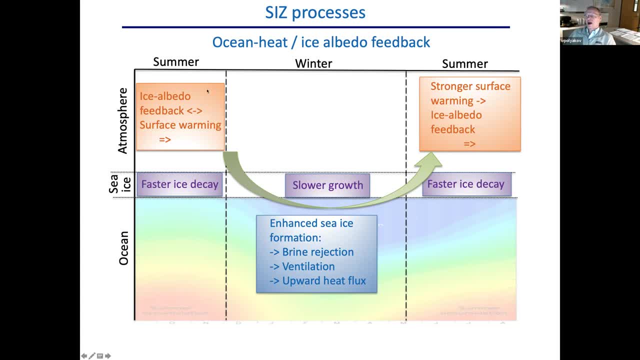 let's go through the seasons. summer we have our cellb, the feedback when surface warming, sunfec and tienen a like this layer, and that leads to faster ice decay. Faster ice decay is translated in winter to more sea ice formation. More sea ice formation means more colder water, more salt rejected into the water, more. 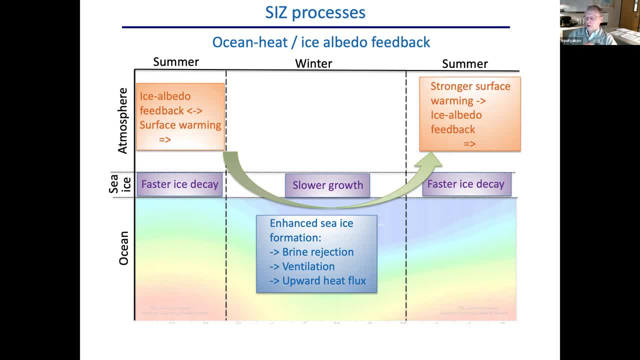 mixing- and that's a component of mixing scheme I was talking about, based on our mooring results. So, based on this enhanced increase of loss of stratification, we expect stronger ventilation of the upper ocean and a stronger upper heat, which reduces the rate of sea ice formation. and next summer comes and the reduced sea ice produces. 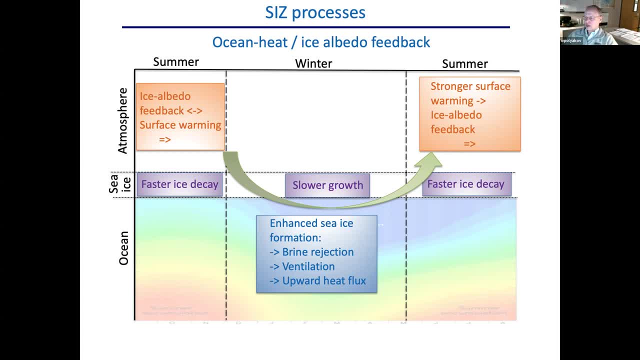 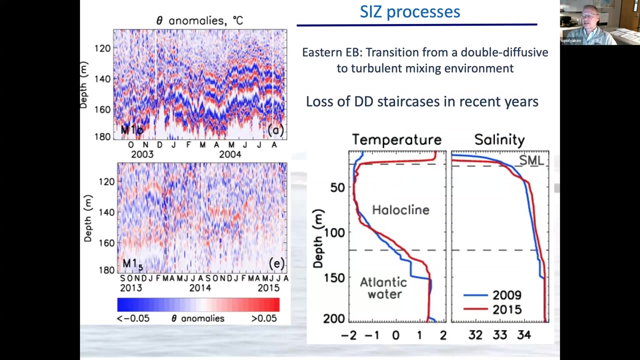 conditions for stronger surface warming and the stronger ice albedo feedback. So we can build this picture Of much stronger feedback mechanism. we were together with ice albedo. we see the work of ocean heat feedback component. These are not only changes in the system. We definitely see. 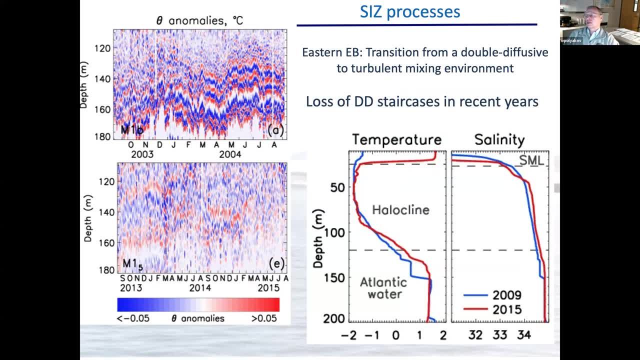 changes with the structure of the ocean in the Eurasian basin. The structure of the ocean. the Arctic ocean was famous in the world due to its very particular feature- step-like structure- and this profile of temperature and salinity for 2009 definitely shows steps associated with double diffusion. 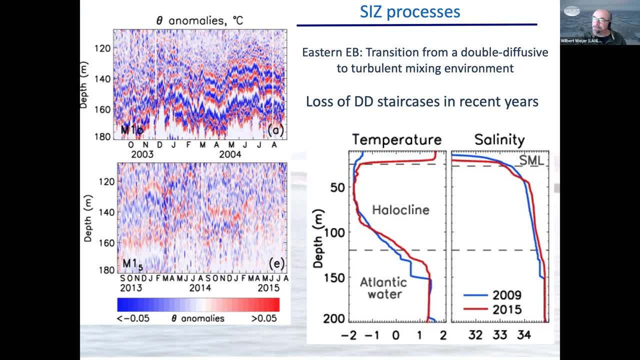 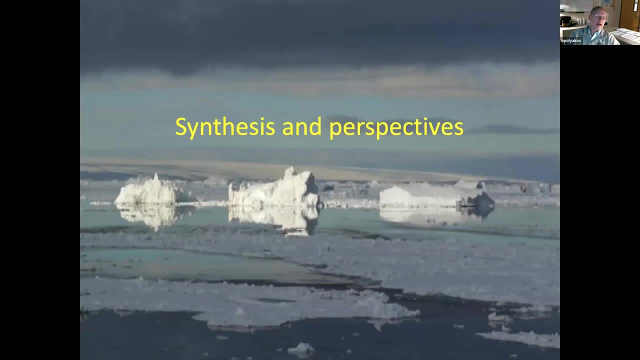 Igor, Yes, Sorry to interrupt. You're at the 20 minute mark, Wondering if you could wrap up so that we can have some time for discussion. Okay, okay, okay. So we have a lot of evidences of the changes in the system and let me jump to synthesis and perspectives. So I would like to show you this. 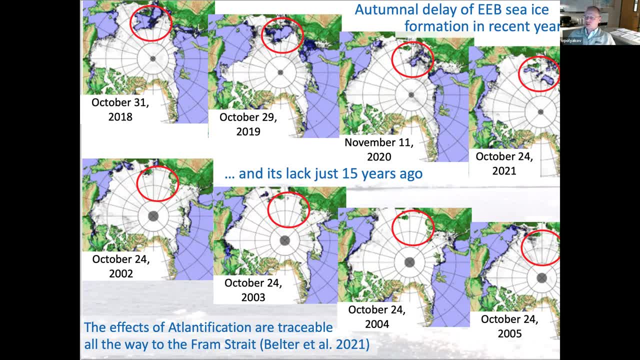 plot which shows, which compares sea ice concentration for four years in 2000s versus four years in 2010s- late years- and we see a difference in ice concentration in the eastern Eurasian basin. This is the beginning of the fall season, sea ice formation and. 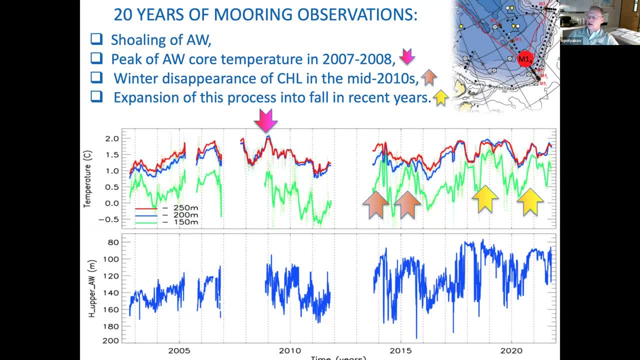 what I was talking about was associated with late release of oceanic heat in later period of time, but what we see here is that this release of of heat happens in the recent, in more early period of time, and we just recovered a mooring from this location and definitely see the big changes in the system where the mixing in the system starts. 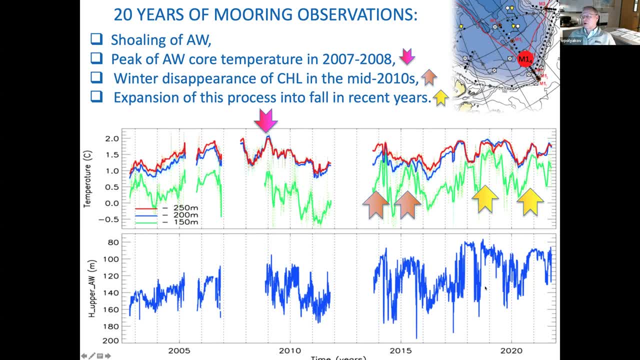 in much earlier, in October, November, which may cause this- observed a loss of sea ice concentration in the eastern Eurasian basin. So we definitely see the continuation of the story of identification and changes in the Arctic Ocean. So let me skip this plot and jump to. 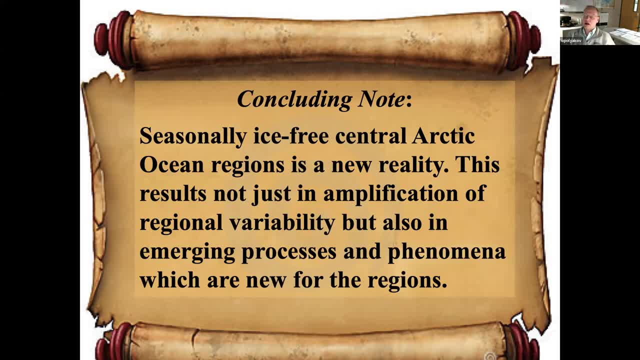 my conclusions that seasonally ice free central Arctic Ocean regions is a new reality and this is a not just amplification of regional variability we observed in the past, but there are some emerging processes and phenomena which are new for the regions. So we are talking here about a really 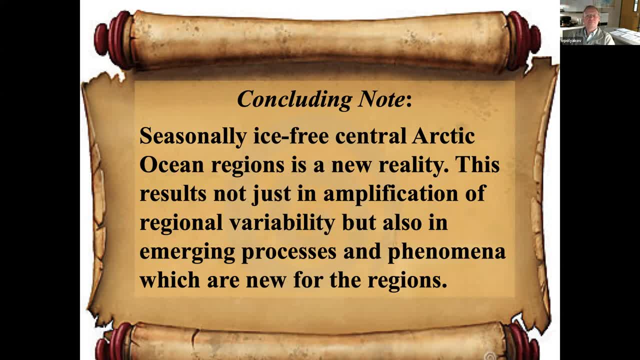 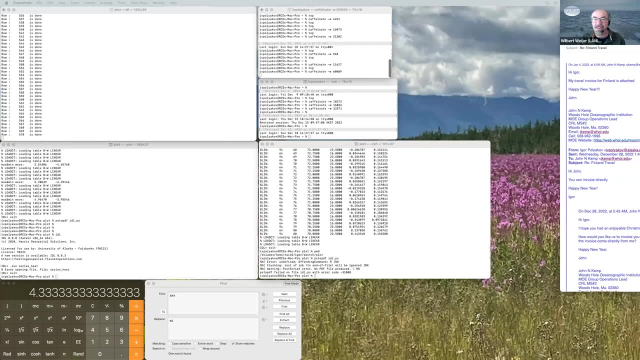 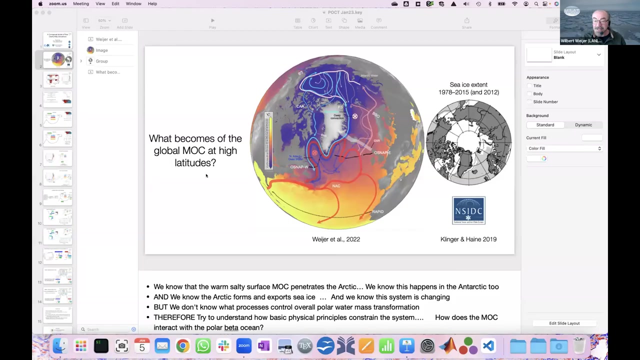 new Arctic. Thank you very much, Awesome. thanks so much, Igor. Extremely interesting presentation. In the interest of time, I propose that we move on to Tom Haynes presentation and reserve the the response to the questions for after that presentation and the discussion. Excellent so, Tom. Professor for Earth and Planetary Sciences at the Johns Hopkins. 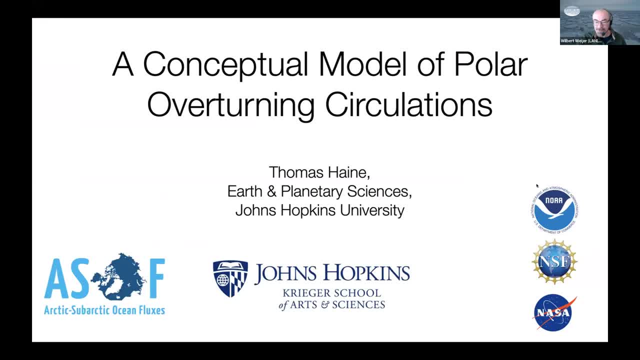 university and he will talk about the conceptual model of polar overturning circulations. Okay, can you see the screen, folks in the cursor? Yes, we can. Okay, fantastic. so thank you everybody, Happy New Year. Thank you for the invitation. So I want to talk about conceptual model of polar. 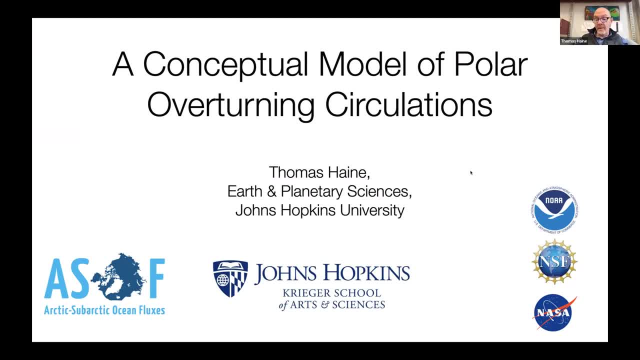 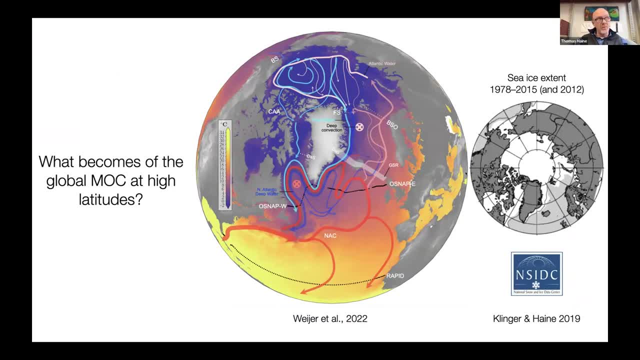 of polar overturning circulations, and I'm gonna talk specifically about the Arctic. There we go. Now we know that the Arctic receives warm, fresh water from lower latitudes, and then interaction with the atmosphere creates the water masses that Igor's just been telling us. 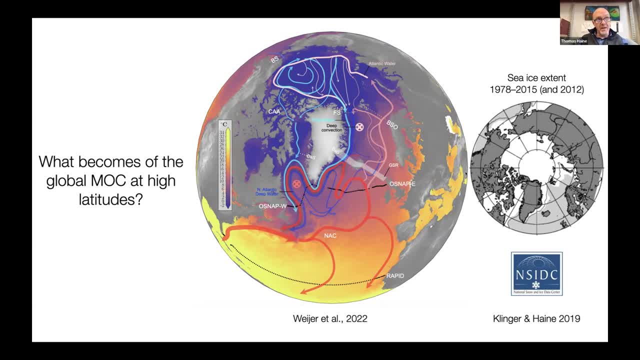 about, in particular, sea ice and polar water, But we don't know the water mass transformation processes that control that conversion of warm salty water into polar water And therefore it's important to try and understand the constraints on the system from basic fundamental physical principles. 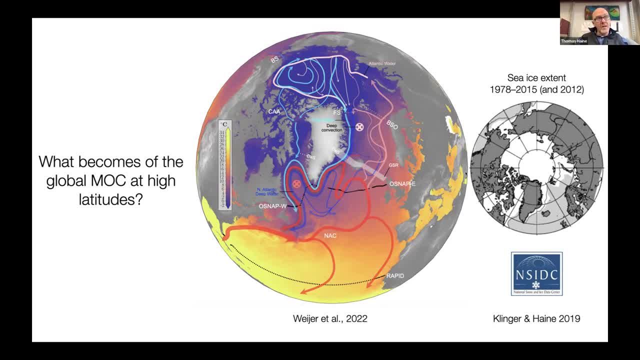 and that's what I'm gonna try and do today. So when I'm talking about the polar oceans, in fact, what I really mean, what I really have in mind, is the beta ocean, in other words, the part of the ocean where there is strong halocline and there's surface sea ice. 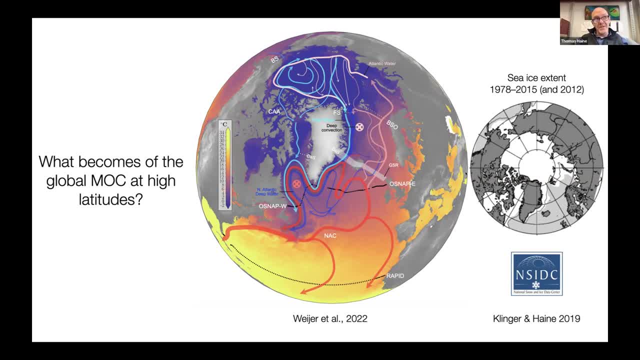 So in today's climate, polar ocean and beta ocean are kind of synonymous, but you should distinguish, at least conceptually, that they might be different, And so the overarching question is this on the left: what becomes of the global overturning circulation at high latitudes? 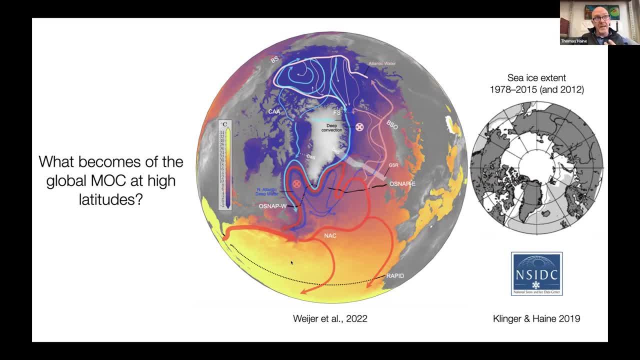 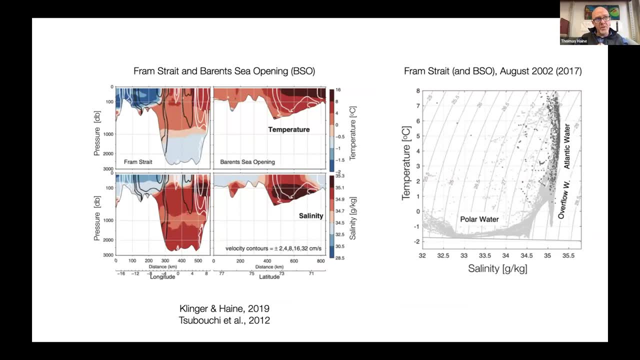 The focus is gonna be on the Arctic, but a lot of what I'm gonna say at least has qualitative relevance to the Southern Ocean as well. Okay, so let's look at the water mass structure for the waters exchanging between the Arctic Ocean and the Nordic Seas across Fram Strait. 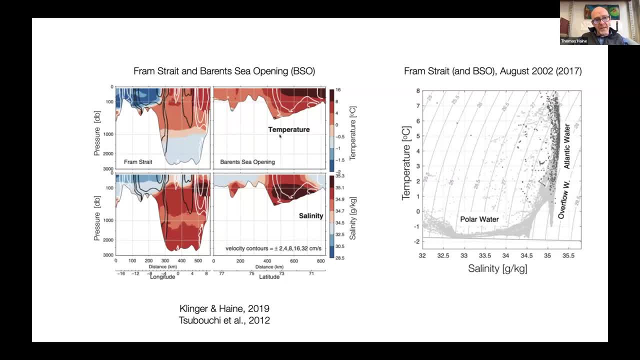 and the Barents Sea opening And you can see on the left-hand side temperature and salinity, and then the contours are showing the speed of the current. So white means into the plane. So this is the warm, salty Norwegian Atlantic inflow across the Barents Sea. 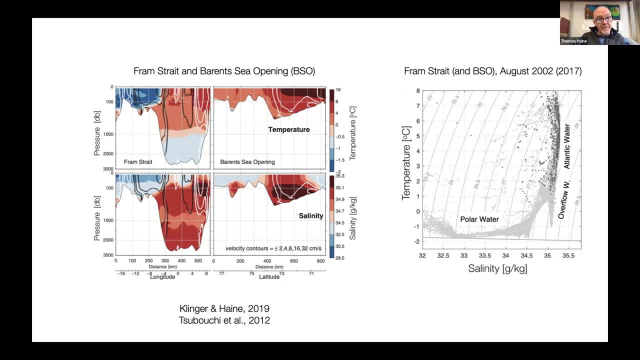 This is the West Spitsbergen current, And then the outflow is on the Western side, the polar water, which is at the freezing point and very fresh, And then there's a deeper branch of the East Greenland current, which is actually not all that dissimilar. 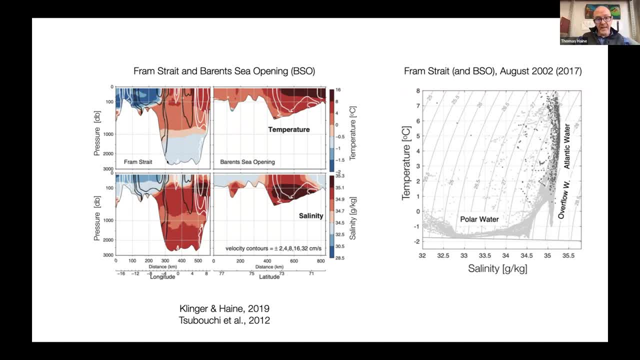 in temperature to the inflowing water. It's a little cooler and it's a little fresher. And so in the TS diagram we see inflowing Atlantic water here and outflowing polar water And then the deep part of the East Greenland current. 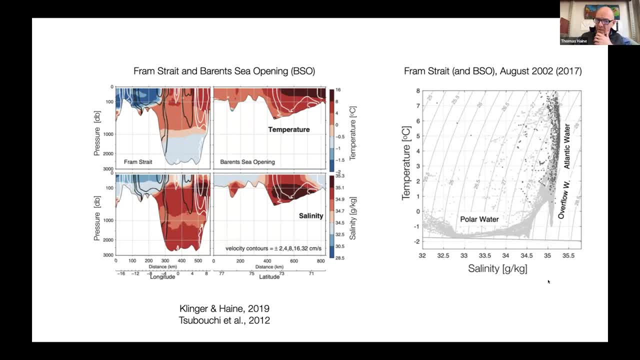 is what I've called overflow water here, So the system you can think of as receiving warm salty water. in the Atlantic water inflow There's heat loss to the atmosphere. The atmosphere deposits fresh water on the surface, either directly by precipitation or via runoff. 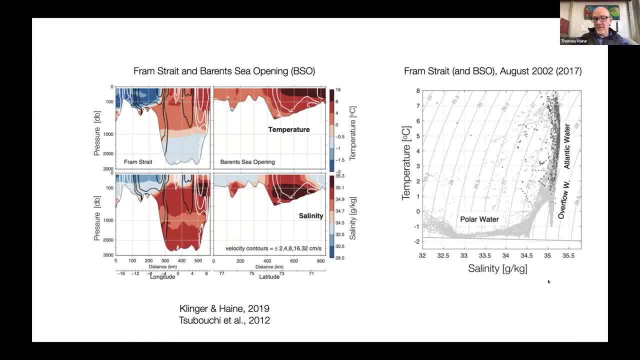 And the system produces three different types of water mass. So one of those is the polar water, So it's at the freezing point, at the surface, very fresh. Another one is the overflow water, cooler, slightly fresher version of Atlantic water. 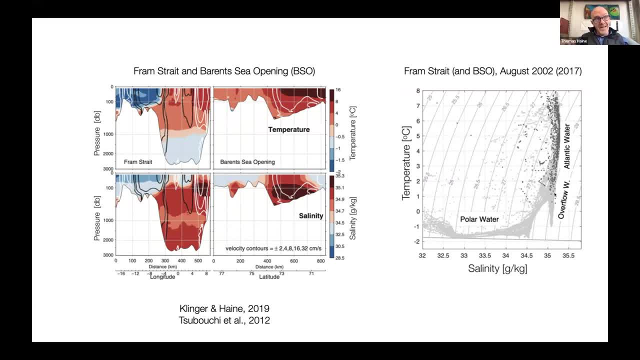 And the third one is sea ice. The question is: what determines the relative proportions of those three water masses- Atlantic water- in these three different modes out? What controls how much overflow water, how much polar water? And so that's the question I'm gonna try and tackle. 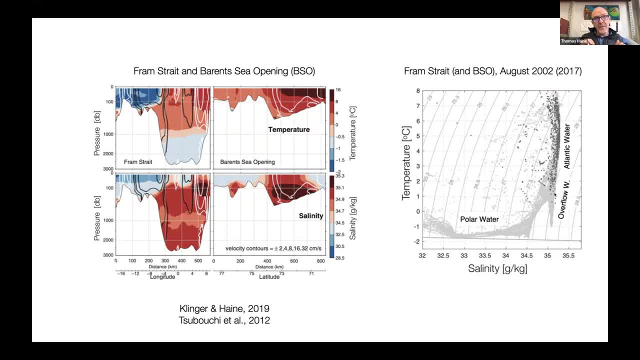 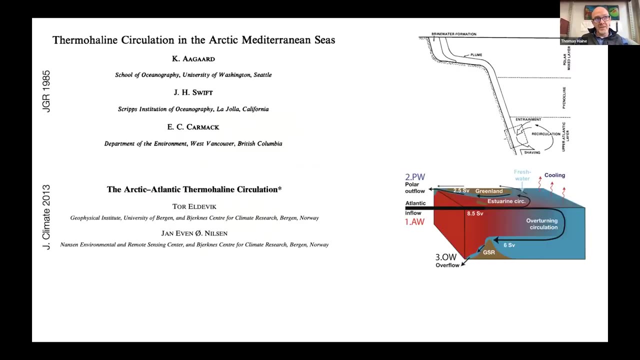 in this talk, with this conceptual model, And I'm gonna apply basic physical principles, in particular conservation of mass and salt and heat, plus a few other conservation principles, to try and constrain those water mass transformation processes. Now we have to be somewhat prescriptive. 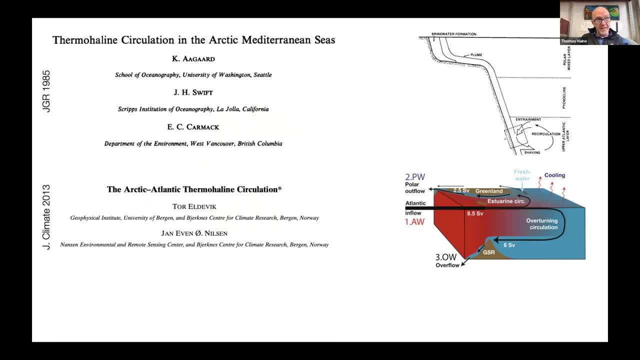 in deciding how those processes can work, And so I'm guided by a few key papers here, And the first one is this paper by Agar et al from 1985, which emphasizes the role of the shells. So on the shelves you can have net sea ice formation. 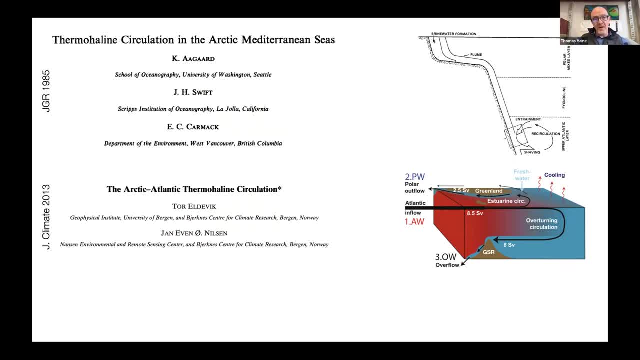 Sea ice is exported from the shelves by the winds into the deep Arctic And by the process of sea ice formation. the water gets salty and brine is rejected, which makes the and the water is at the freezing point can convect all the way to the bottom. 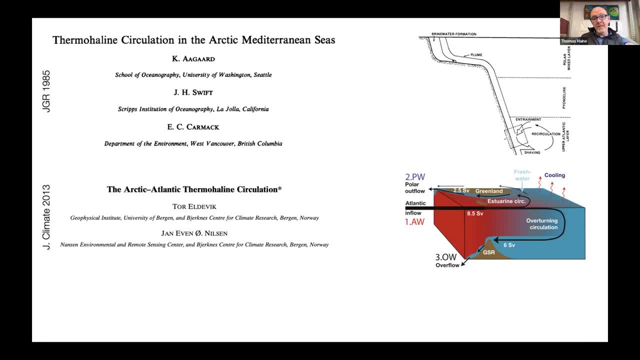 which makes a very dense, saline, briny shelf water And that can overflow into the deep ocean And as it overflows it mixes, entrains the ambient waters. So you can see this entrainment process And in fact, in this particular example, 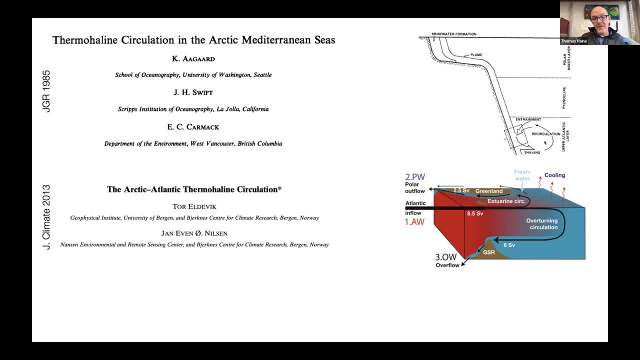 it's going beneath the picnic line on the upper Atlantic water layer. Okay, so this is a fundamental way in which extraction of heat from the Atlantic water can form sea ice- where there's net export of sea ice from the shelf- and also form this overflow water. 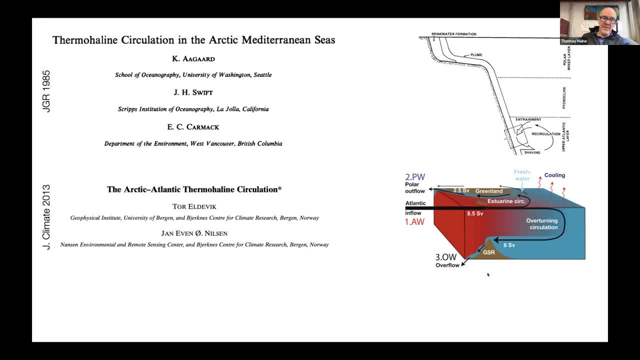 And then the other paper which is particularly useful is this paper by Tor Aldavik and Janneven Nielsen from about 10 years ago, which was looking at the same kind of system but in a somewhat different way. They were thinking about the Greenland Scotland Ridge. 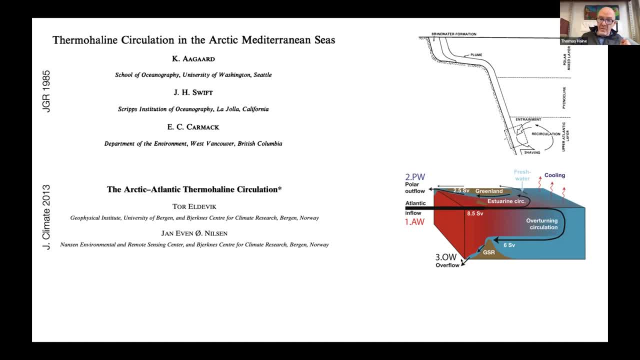 Atlantic water inflow formation of one branch- overflow water, thermohaline overturning cell, and then the other branch, the polar water, which is sometimes called estuarine circulation. Okay, so let's think about their model a little bit more. 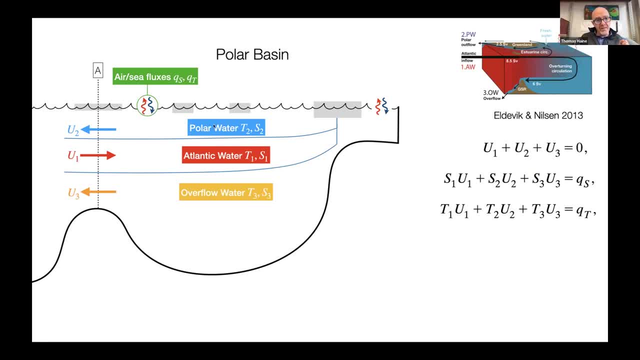 They have Atlantic water flowing in air-sea interaction. polar water flows out at the surface, overflow water flows out at depth beneath the inflowing Atlantic water, And what Aldavik and Nielsen do is they construct a volume budget and they construct a salt budget. 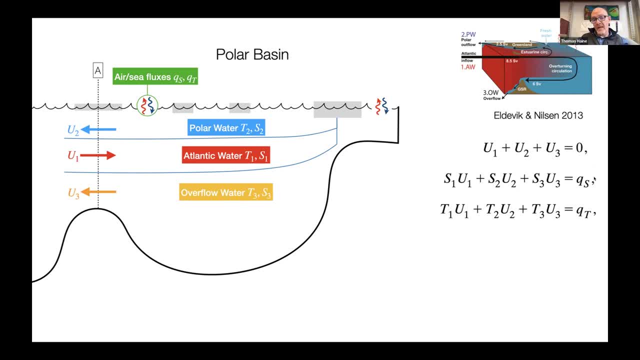 and they construct a heat budget. So QS and QT are the net air-sea fluxes of salt and heat And this is a system that has these constraints, that will conserve these different quantities. Now there are some deficiencies or issues with their model. 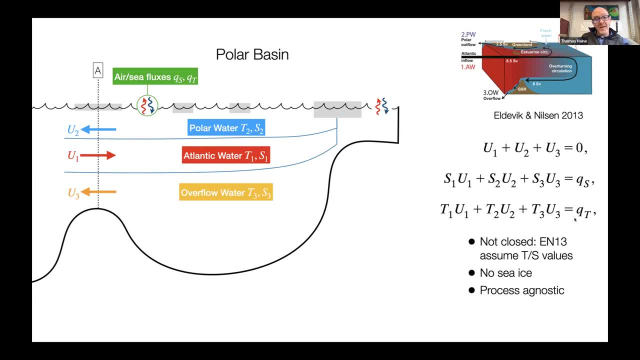 And, in particular, this system of equations isn't closed. So, for example, if you specify the Atlantic water inflow strength and its properties and you specify the air-sea fluxes, you can't determine uniquely what specifies the amount of polar water or the amount. 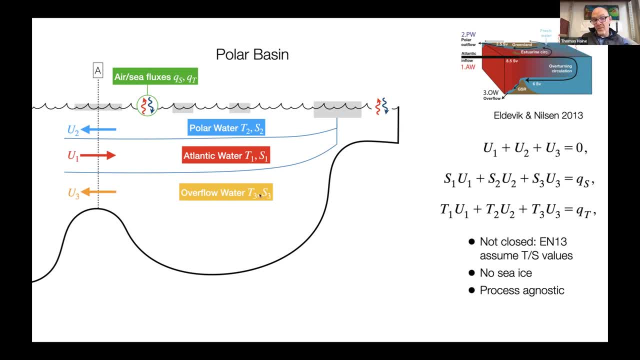 of overflow water coming out, because you need to also specify their temperatures and salinities. Okay, so the way that Aldavik and Nielsen got around, that is, they assumed reasonable values for polar water temperature, salinity and the overflow water temperature, salinity. 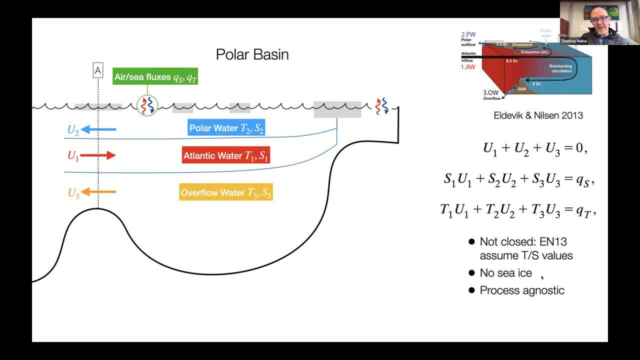 That's undesirable. The other thing is that they don't have any sea ice, So a key part of this process is missing- formation of sea ice- And it's also process agnostic: It simply specifies a budget of these various different quantities. So I wanted to be a little bit more prescriptive. 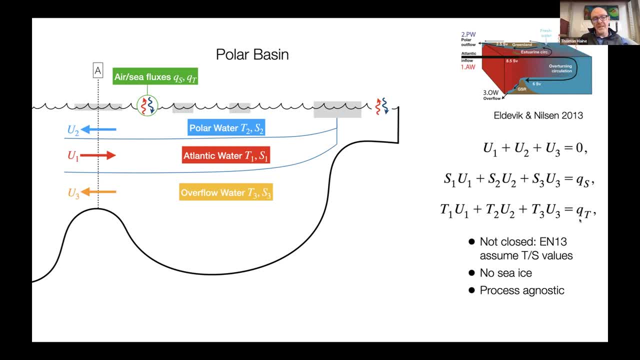 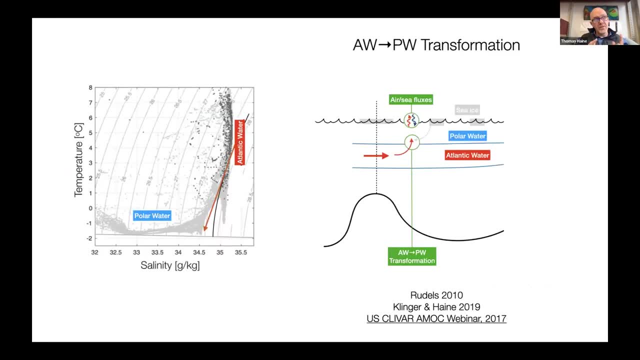 in specifying processes that will convert Atlantic water into polar water and into overflow water and get around some of these restrictions. Okay, so let's talk about the first process. The first process is Atlantic water to polar water, So the Atlantic water, which is the flora and fauna. 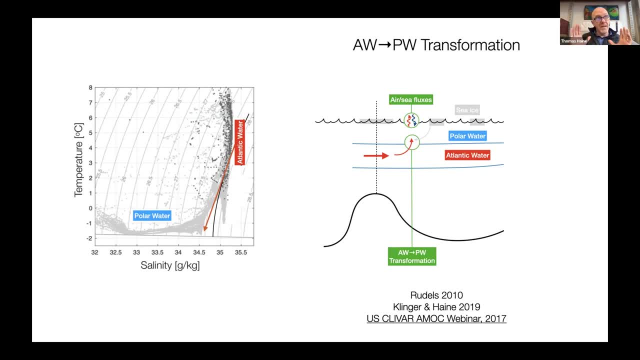 that holds, see ice down in polar water is a polar polar coated sea ice. Rather than like a valeur value, the sea ice could be Te derivation Seven. So polar polar covers and then the Atlantic water covers the Earth. The Dual polar polar covers the river. 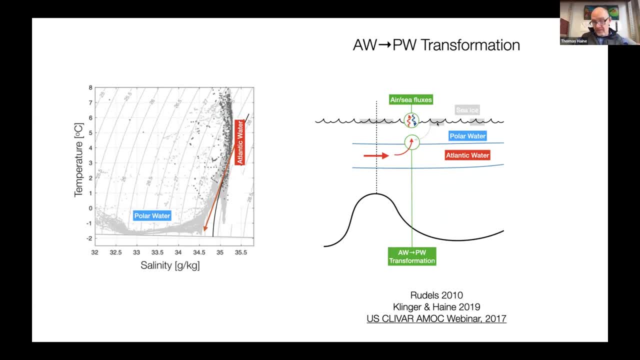 This houses the sea and 하니까 may have water and some similar kinds of water, and remember, this is the center of the hemisphere. They're eggs, Perfectly. water is cooled- it has to be cool to the freezing point- and it's freshened. it's freshened because 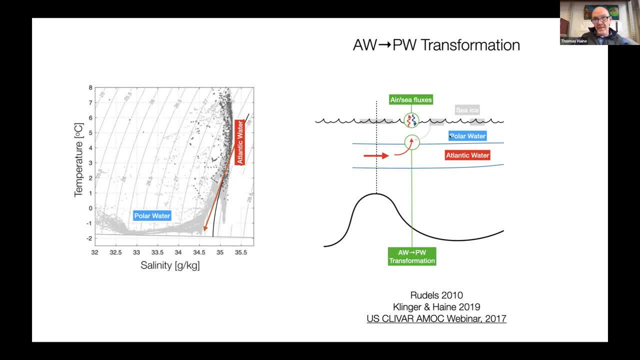 it's melting the sea ice and that will produce a surface buoyant layer which is fresher at the freezing point, and so that is formation of atlantic water. and so in the ts space you're going from atlantic water down to the freezing line here. into fresher silences now, in order for 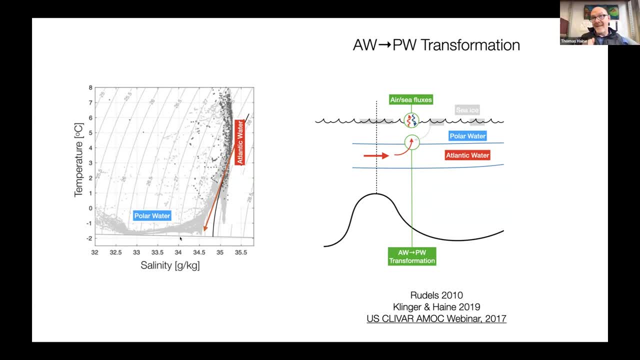 the polar water always to be less dense, more buoyant than the atlantic water. in this process, you can only travel in the ts diagram along this red arrow or to its left. okay, so what is this red arrow? so i'm starting from some atlantic water ts. 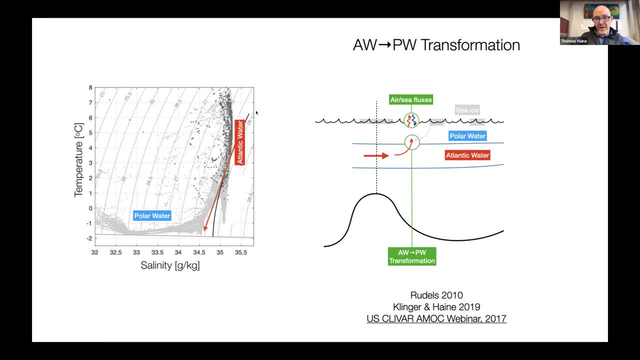 point up here and this red arrow is the tangent to the isopignol that passes through that point. okay, so if i'm freshening more than i'm cooling, then i'm going to create a less dense, therefore more buoyant, polar water, and you can see from the ts diagram in the fram straight. 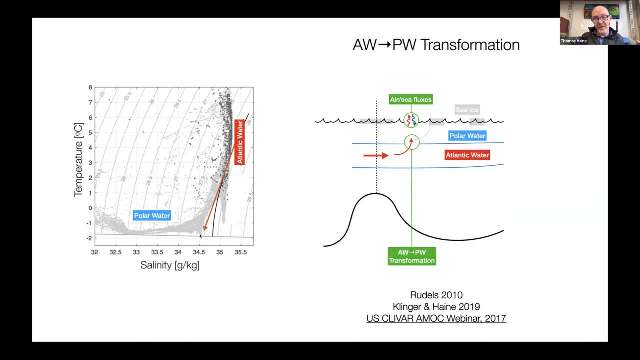 there's this very hard sharp upper limit to the salinity of the polar water, which is a little more than 34.5 here. okay, so i'm claiming that that is because there's this tangent line from the atlantic water. if you're going to make polar water from atlantic water by mixing with sea ice, 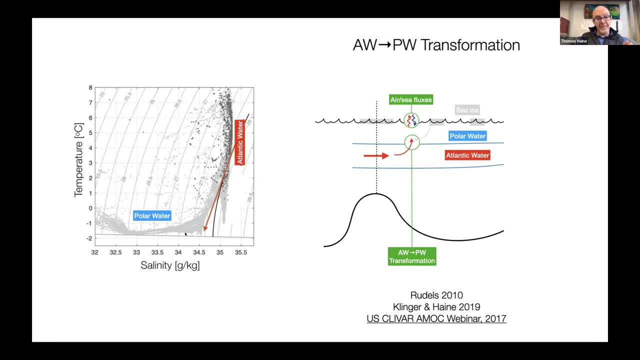 cooling and freshening. you can only ever be to the left of this red line. oops, sorry. okay, so that that is one of the. that is one of the key mechanisms. now, um, i'm not going to show you many equations at all, if you're interested in more details. um, burt rudels talks about this in: 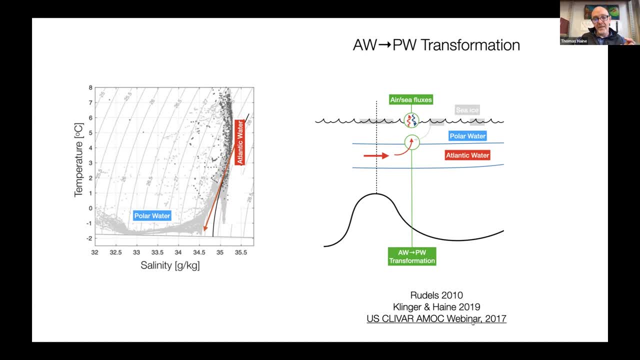 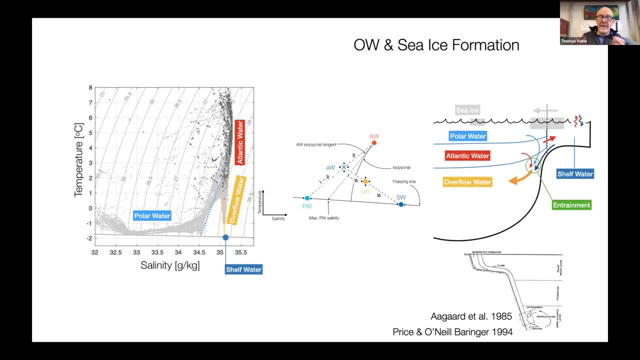 a nice paper from 2010. it's in, it's in this reference, and there's a webinar which you can go to. you can click this link and you can see me talking about this in more detail there too. now, the second mechanism of atlantic water is the salinity of the polar water, so if you're going to 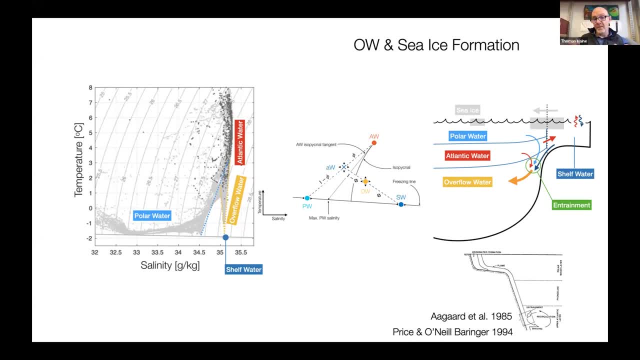 look at the lij's Prona xxx on the right you can see there's one uh angle between the sait and the heel that will be directed to the flat ice score hundred of years to arrive and where the salt begins to 1918. kid, not prevent if the salt is only three. know the interaction. atlantic water. 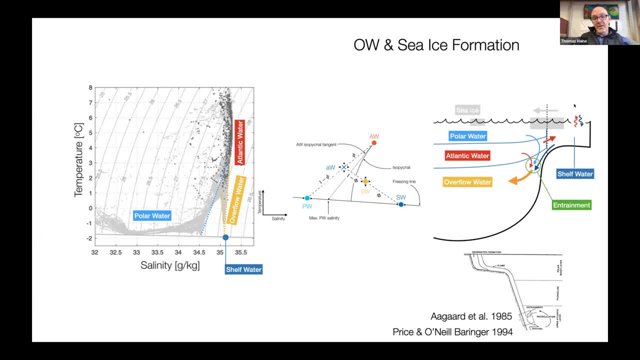 conversion is the shelf interaction, and in fact there's there's more than one piece going on here. so let's start up on the right with this schematic. so we have the shelf water, and i have in mind this ar Spotify in the background, in part because, in the making of these, Civilę Est delve into the 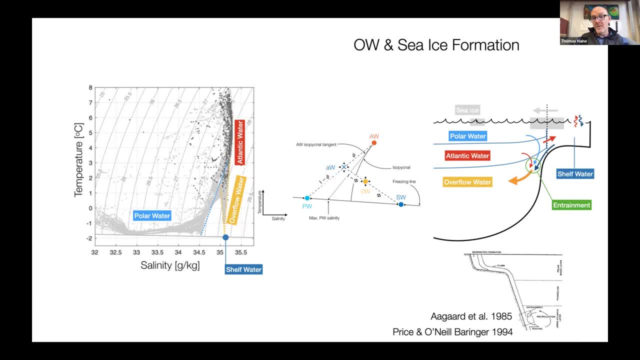 view, atlantic water penetrates onto the. if it loses heat to the atmosphere, it maybe gains some fresh water, for example from runoff the it into the deep basin, then ultimately into low latitudes. the water that's left behind on the shelf gets briny and therefore more dense, and eventually it overflows. as it overflows, it entrains. 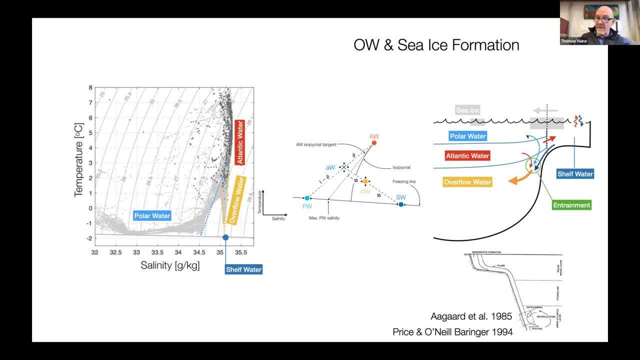 ambient water. and the ambient water consists of a mix of the water masses that are hanging around near the shelf break, which are polar water and atlantic water. okay, so some of the atlantic water gets up onto the shelf and then is modified by the shelf processes. some of the atlantic water 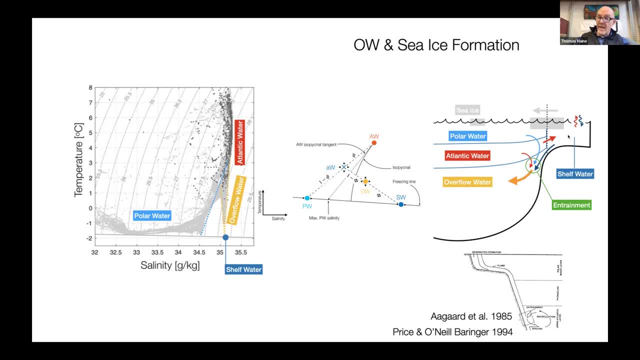 gets entrained directly into the overflow without ever being exposed to the atmosphere on the shelf. okay, so let's look in ts space at how that works. let's look at the data plot on the left to begin with. so we're starting here with atlantic water, here's the polar water. what i'm saying is that 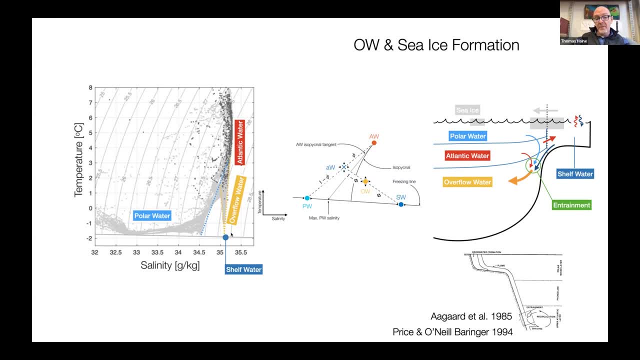 there's another water mass which is not on this diagram, which is shelf water. so that's at the bottom of this diagram, which is shelf water. so that's at the bottom of this diagram, freezing point, and it's salty, it's saline. okay, so here, for example, would be: uh, where shelf water? 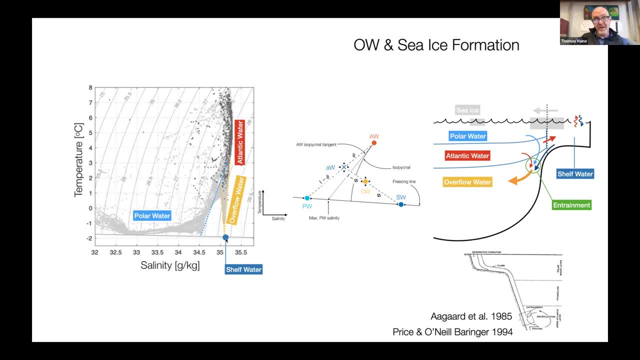 would exist. now the data are from fram straight and balance the opening, so there's no surprise that there's no shelf water water mass of these characteristics, uh, in those data. anyway, here's this shelf water water type and it mixes as it overflows with the ambient water. so the 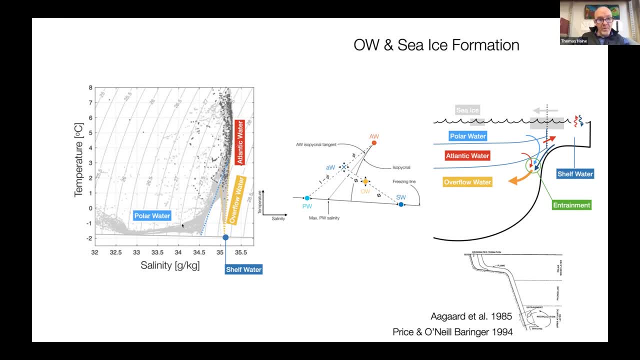 ambient water is going to be along a mixing line between polar water and atlantic water. shelf water mixes with those and it forms this overflow water mass with these characteristics here. so it's cooler and slightly fresher, okay, and then in in a schematic ts space. here's the shelf. 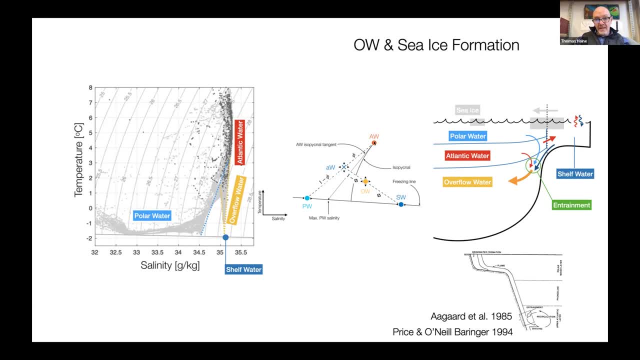 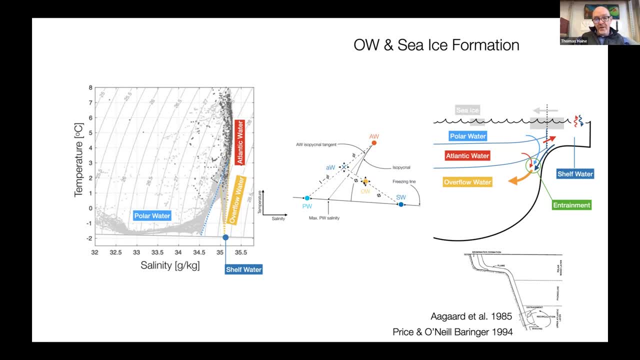 and then a mixture of those two which form ambient water. the overflow water is formed by a mixture of the shelf water and the ambient water, and that mixture is controlled by this greek capital, phi, which is the entrainment. so if entrainment, the fractional entrainment is large. 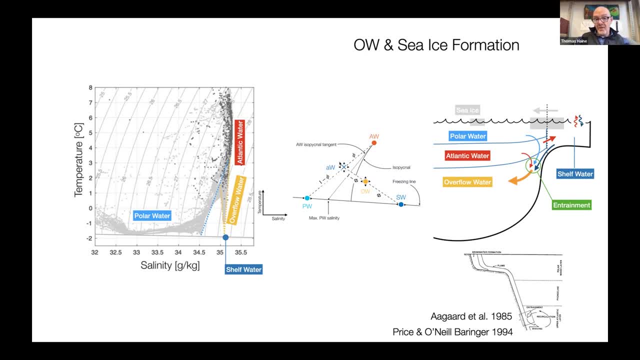 then the overflow water properties are close to the ambient water properties and most of the atlantic water goes straight into overflow water rather than going to the shelf, and vice versa. okay, so entrainment can slide this overflow water ts properties backwards and forwards along that dashed line. okay, so now let me put these elements together for you and show you. 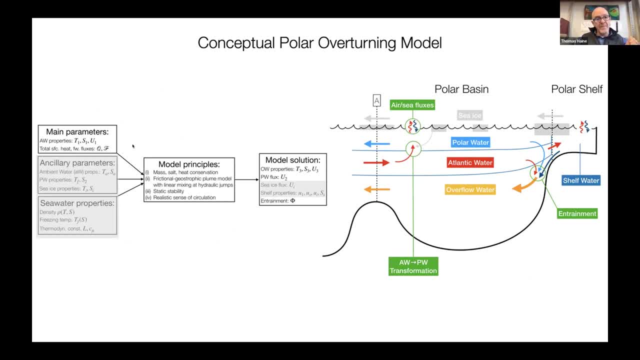 some results, so i'm skipping lots of details here. you can ask me if you have questions or look at the references. the main parameters that go into this model are the atlantic water properties, so it's flux, it's temperature and it's salinity, and then one specifies the total amount of heat lost. 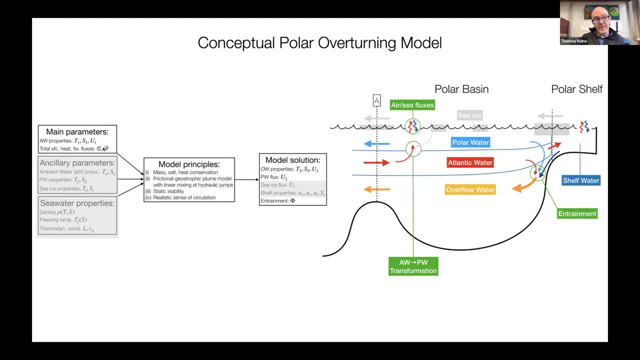 from the ocean to the atmosphere and the total amount of fresh water exchanged as well. so it doesn't matter if that's coming from precipitation or runoff. okay, there's some ancillary parameters which i'm not going to talk about. the model principles are: you conserve mass salt and heat. 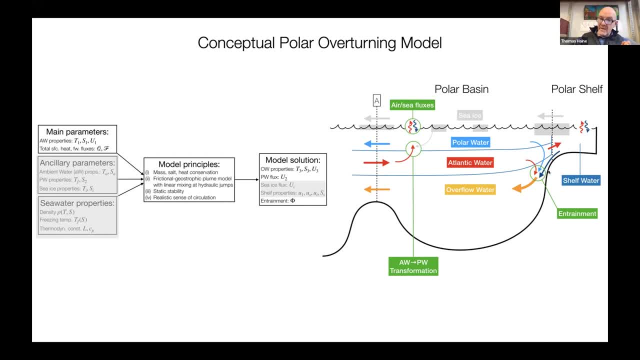 you have a specification for this entrainment parameter, this capital phi? okay, and that is a frictional geostrophic plume model with mixing hydraulic jumps, based on some of the work from overflows by Molly O'Neill, Berringer and Jim Price. We require the system to be statically. 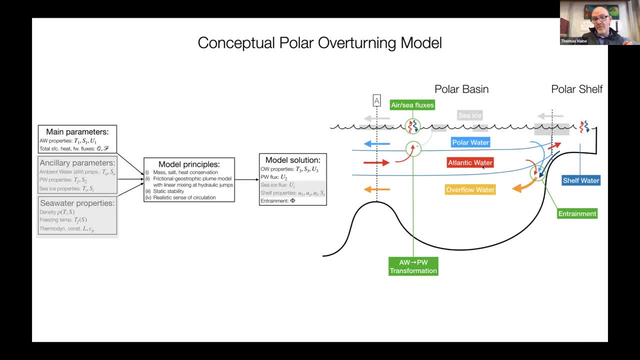 stable. So, in other words, if we have a polar water density which is greater than Atlantic water, that's not an allowable solution And we want a realistic sense of circulation. In other words, Atlantic water flows in ice polar water and overflow water flow out, If the system is. 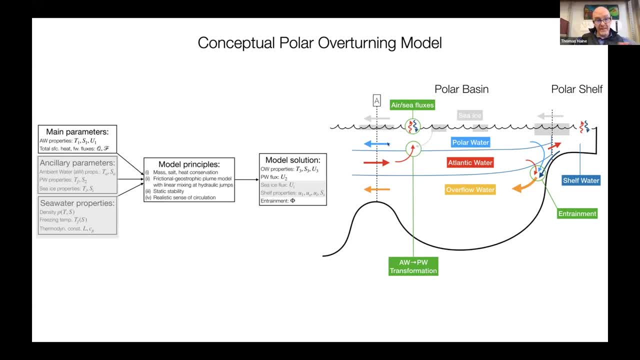 saying, hang on, I need the polar water to change its direction, then that is also not a legitimate solution. So what comes out of the solution of this are the properties of the overflow water, its temperature, salinity and its flux. the flux of the polar water. the temperature of the polar 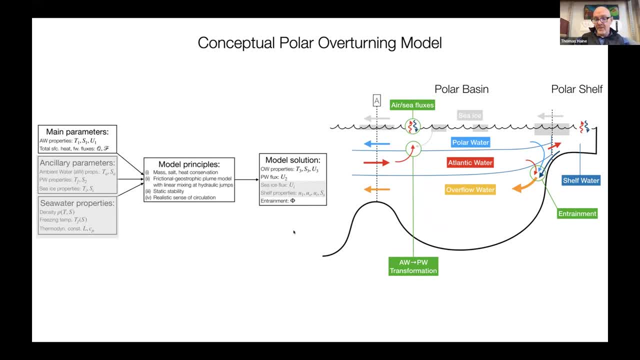 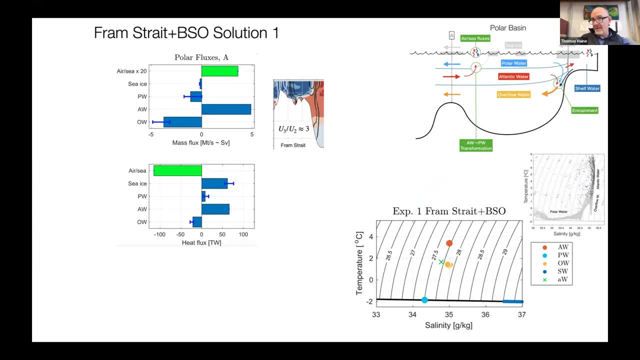 water is set at the freezing point and the fractional entrainment rate. Okay, so let me show you some solutions. So this is a canonical solution that is in the moderately realistic parameter regime And it shows on the top diagram the fluxes, mass fluxes, okay, but you can think of it as 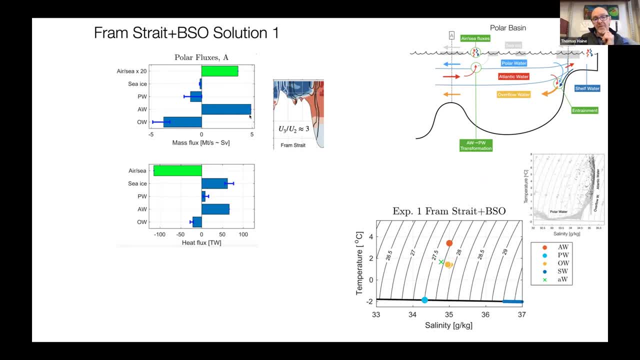 sphere drips. Here's Atlantic water: about five sphere drips flowing in in total. The system: it gains some fresh water from the atmosphere. it loses heat. it produces three water masses: sea ice, polar water and overflow water, And this particular solution has about three times. 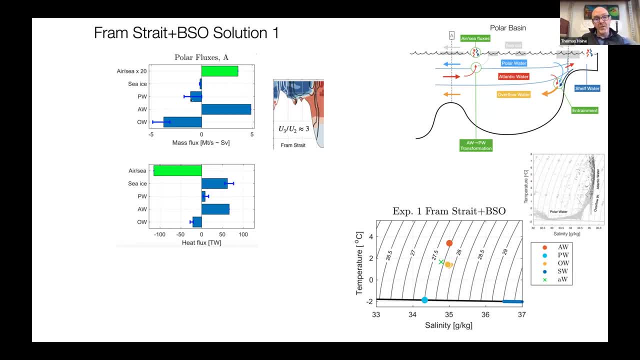 as much overflow water being produced as polar water, And that is moderately realistic. If you look at the fluxes across the Fram Strait, polar water is about a third as much as the East Greenland current. Okay, the vertical scale is stretched here, so it doesn't look like it's one third as much. 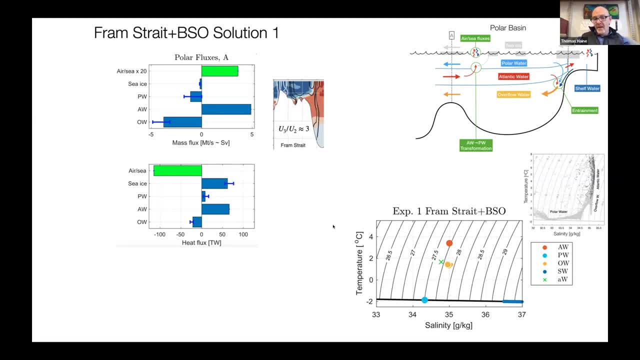 Okay, and let's- let's skip the heat flux diagram for the moment. Here's the TS space. you have a very saline shelf water and you have a lot of entrainment, So the overflow water properties are close to the ambient water. 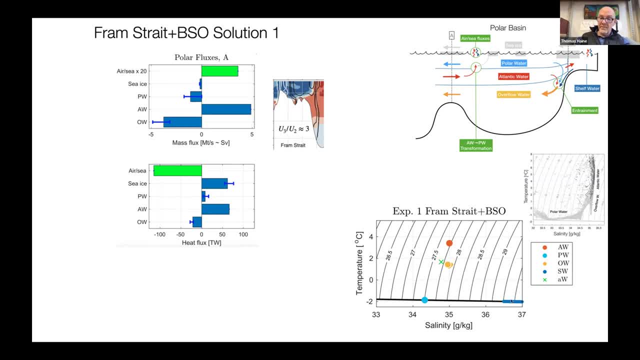 So small amount of salty shelf water overflows entrains a large amount of ambient water to form overflow water, which is therefore relatively warm. Okay, now I'm going to change the heat flux loss slightly. In fact, here I've increased the heat flux by about 20%. 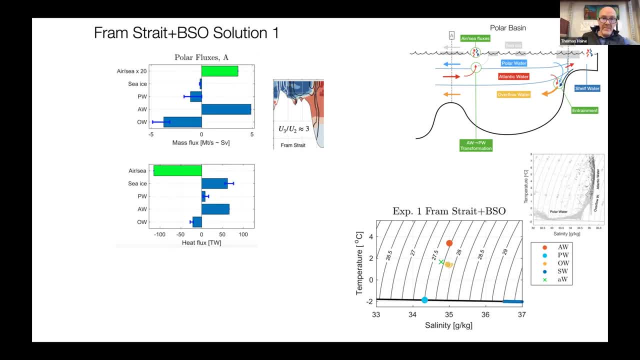 Okay, otherwise everything else is held fixed. Now this upper diagram- you might not have noticed. the upper diagram essentially stays the same. So you still have about 30% of the heat flux. So that means that you can have three times as much overflow water coming out of the system as you have polar water, which is moderately realistic in round numbers. 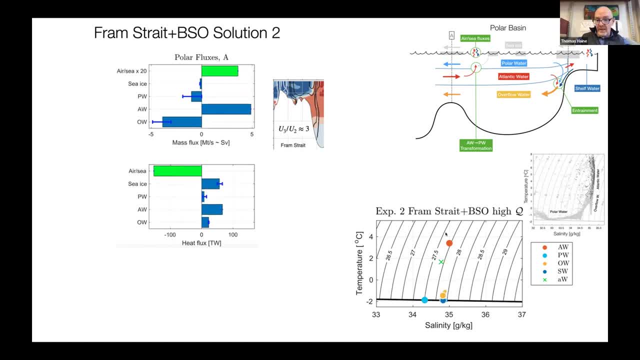 The heat fluxes are different And, more importantly, the TS properties of the overflow water are quite different. So now the overflow water is very cold and it's a bit fresher. It's near freezing, Okay. so same flux, but now it's much colder. 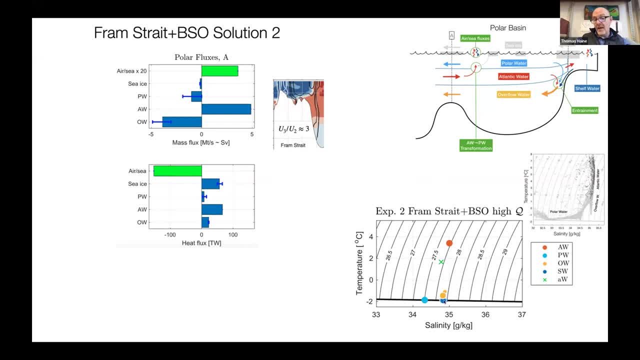 And shelf water is now much fresher. Okay, so the same flux, but now it's much colder, much fresher than it was before. so this is a case where there's very weak entrainment. okay, the overflow water is close to the shelf water, ts properties and the atlantic water in this solution. 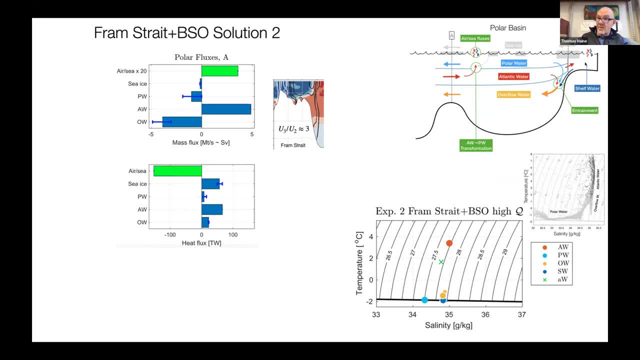 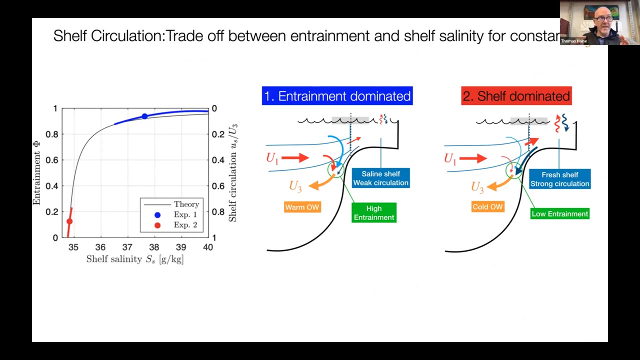 is primarily crossing onto the shelf interaction with the atmosphere, then overflowing is a relatively not dense overflow and therefore undergoing little entrainment. okay, i know, all i did was change the heat flux by increasing it by about 20, i think the number was in this case. so there's a trade-off between this atlantic water being converted into overflow water. 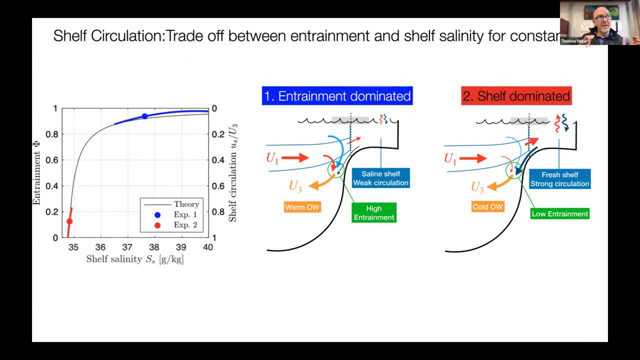 via entrainment, or atlantic water being converted into overflow water via a pathway onto and off the shelf. there's a trade-off between entrainment and shelf salinity. for everything else, held fixed okay. so let's look at that trade-off. so here are the two solutions i just showed you. this is the. 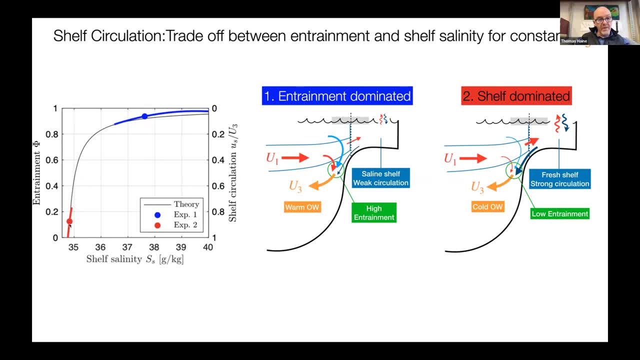 one which has got low entrainment. this is one of the relatively high heat flux. i call it shelf dominated. here's the one with very high entrainment, very saline shelf water and a low, weak shelf circulation. okay, and then there's theory which blinds. these two points up. so the two solutions canonically. 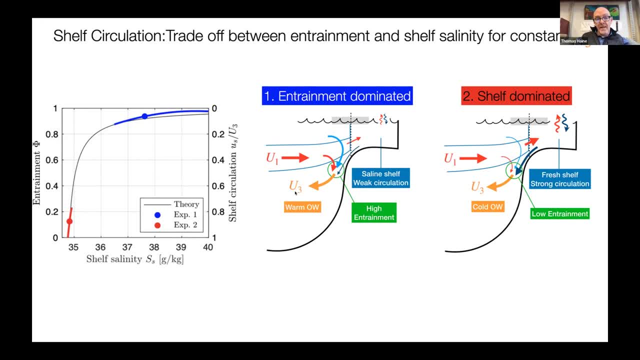 are an entrainment dominated solution where the lenta water gets converted into overflow water directly and there's a weak circulation on the shelf but the shelf is very saline, versus shelf dominated, where the Atlantic water goes onto the shelf, loses a lot of heat, gets cold flows off very. 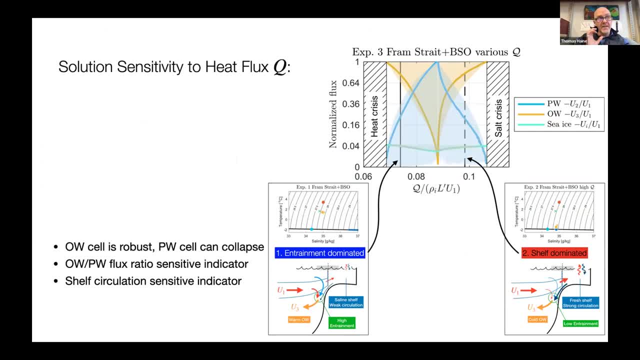 little entrainment. So now let's look at the solution sensitivity to varying that heat flux more broadly. Okay, I've given you two canonical solutions so far, And those two solutions are shown on this diagram by the two vertical lines. So here's the first one. 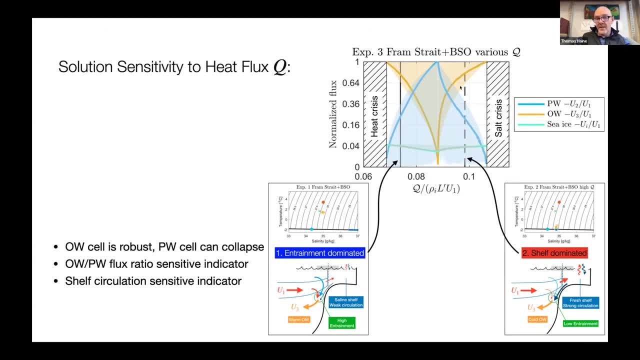 This is the one which is moderately realistic with a warm overflow water. Here's the second one. this is the one which is for the same fluxes but has got a very cold overflow water and the heat loss is a bit higher. So now I've allowed the Q to vary continuously in this range. 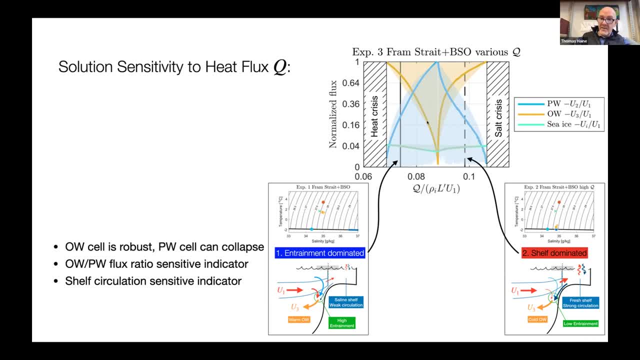 Okay, and what you're looking at here are the various different solutions for the flux of polar water, The flux of overflow water And the flux of sea ice. the system makes these three water masses Okay, so the two vertical lines have got more or less the same: polar water and overflow. 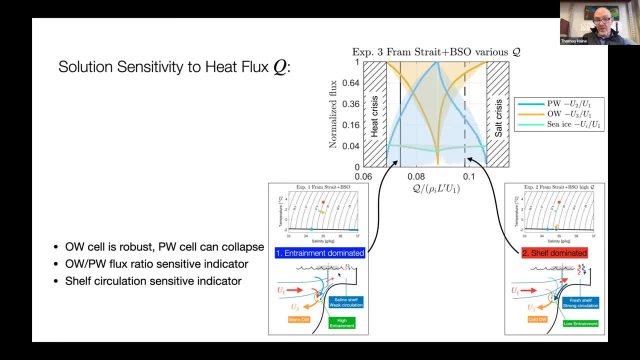 water formation rates, but they've got quite different TS characteristics. Okay, now if I, if I increase the heat flux even more, so I increase it 20% to get to this dashed line, then you eventually reach this point called salt crisis. as you, as you. 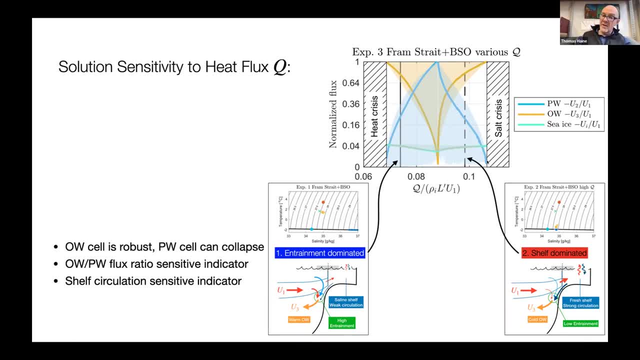 increase the heat loss even more. the polar water gets shut off, it gets weaker and weaker and weaker and eventually it reaches zero. okay, now can't go negative. So when it hits zero, I call that salt crisis and the solution ends. 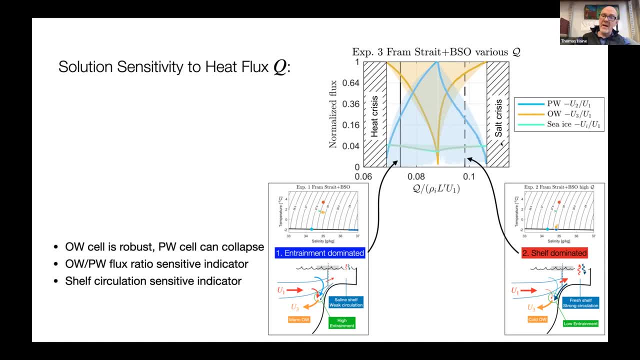 Now, in this particular case, what's happening is the system cannot export enough salt anymore. There's large heat loss to the atmosphere. The outflowing water masses are fresher, Okay, Than the inflowing water mass, and there's relatively little fresh water being added. 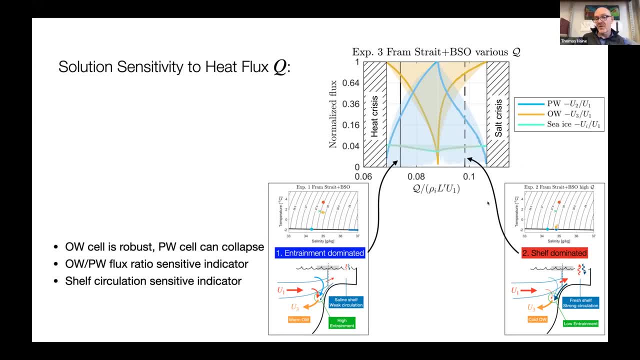 by the atmosphere, And so the system can export the salt that's being imported from the Atlantic water and therefore it This is where the solution ends, in the West. If you went beyond that point, the polar water would change its sense of direction, its flow. 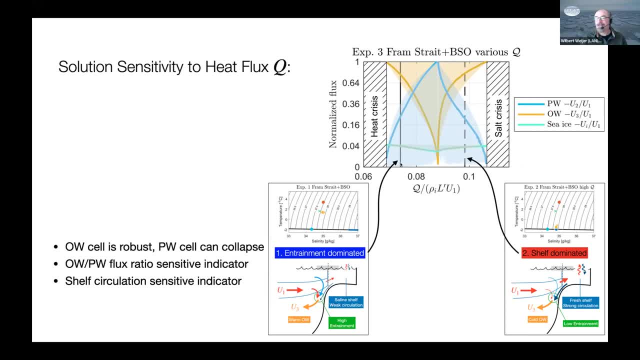 Now, if you start- Yep, I hate to interrupt you with the 20 minute mark- Okay, thank you. Okay, So if you start at this one here and you decrease q, then you reach this alternative thing called heat crisis. Okay, again, the polar water switches off. 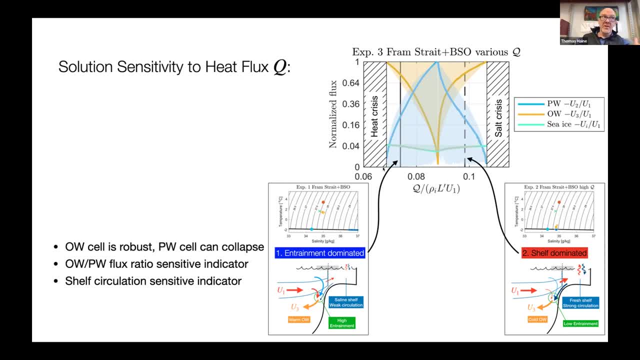 But this is now because the system can't lose the heat in the inflow in Atlantic water. The heat loss to the atmosphere is too weak. Okay, so this diagram shows some, some characteristic things. The overwater cell is robust. in other words, you can- you can always have an overflow water. 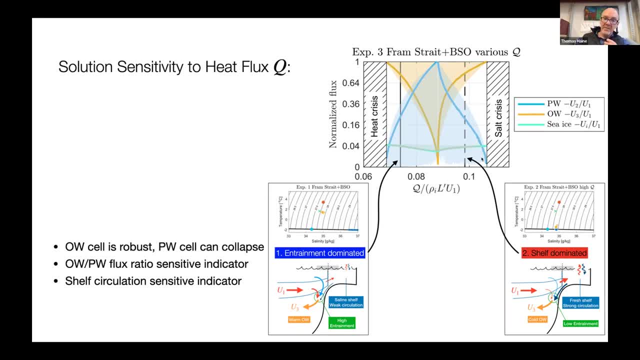 cell, But the polar water cell can collapse. Okay Now q is one of a number of input parameters, So more generally you can vary. also the freshwater flux And then the inflow flux of the Atlanta water is temperature and its saliency. 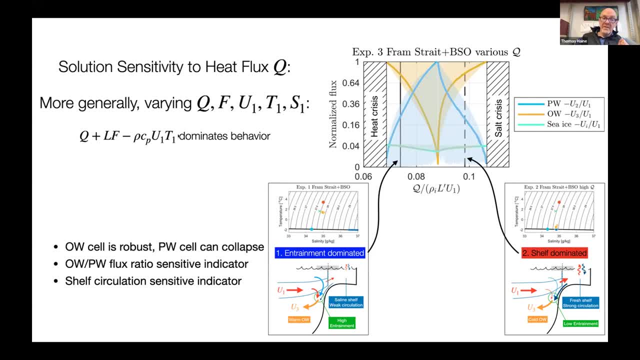 It turns out that the dominant single parameter combination that controls the behavior is this sum of terms. okay, so the saliency of the inflow in water is irrelevant essentially, but you can compensate for changes in q With a change in f or u or t. okay, so let me conclude. 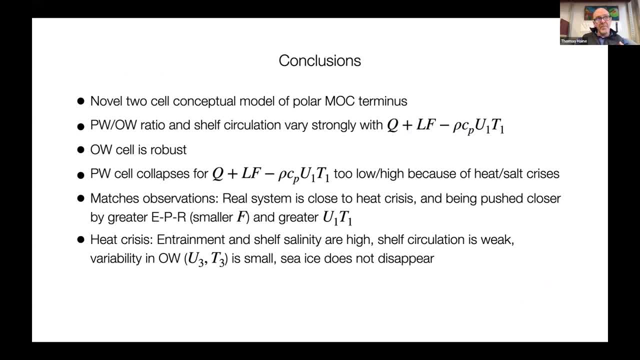 So this is a novel two cell conceptual model of the polar MOC terminus, in particular the presence of sea ice. okay, What it suggests is that the polar flow, the polar water to overflow water ratio and the shelf circulation will vary strongly with this set of parameters. okay, heat loss, freshwater: 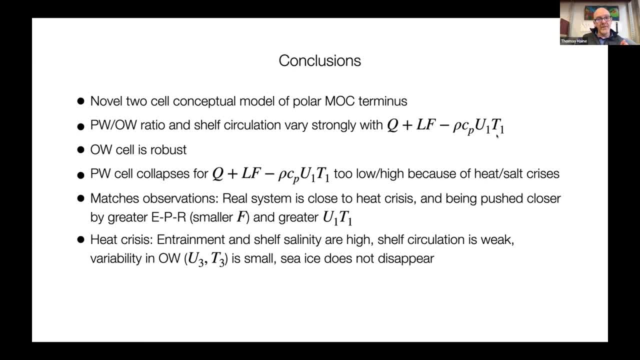 flux and then inflowing Atlanta water. heat flow, The overflow, the presence of the overflow water cell is robust, but the polar water cell can collapse, either because this set of parameters is too high or too low, in what I called a heat crisis, because the system can't export enough heat, or a salt crisis. 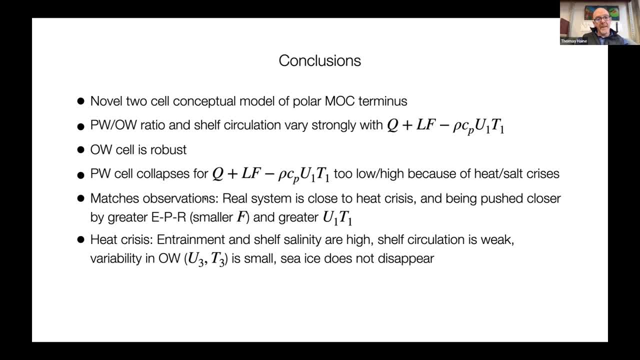 because it can't export enough salts anymore. Now, the one that matches the observations is relatively close to heat crisis. Okay, In other words, if the loss of heat to the atmosphere goes down, or there is more runoff provided from the atmosphere to the water or the inflowing heat flux in the Atlantic. 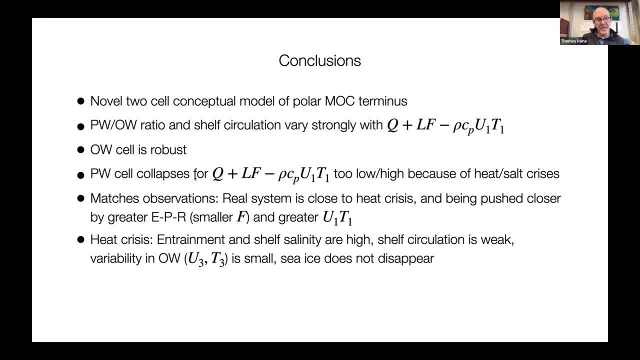 water increases, the system will be pushed closer to the heat crisis and that will be indicated by polar water cell collapse. And as you approach the heat crisis, these are the things that happen, at least in this simple model. Entrainment and shelf salinity are high, shelf circulation is weak. the variability 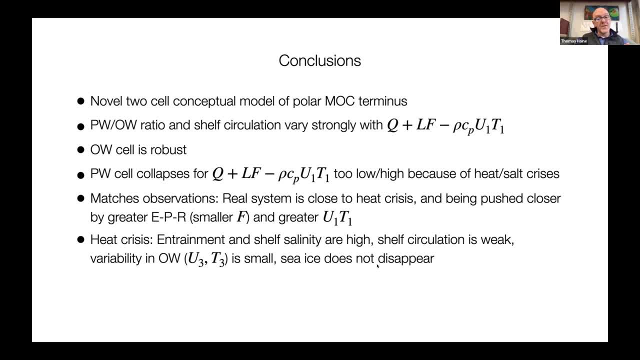 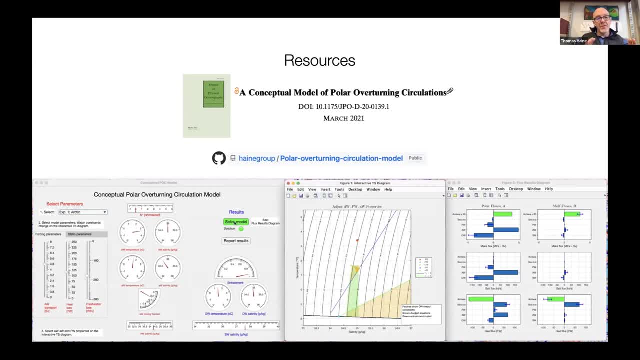 in the system is small and the sea ice does not disappear before the heat crisis occurs. Okay, so that's everything I wanted to say. Here are some resources for finding out more, including some GitHub repos and an interactive app where you can explore this. 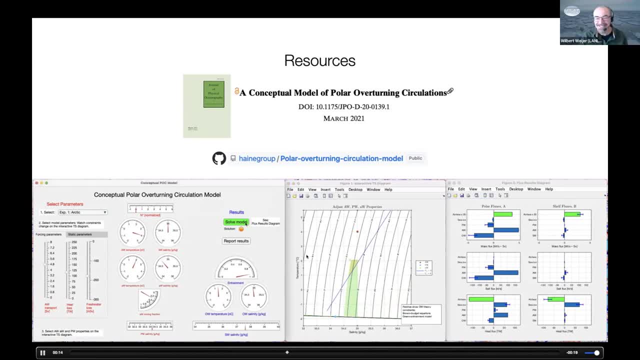 Thank you. Great Thanks, Tom. This is extremely interesting. I'm going to stop here, Thank you. Thank you also for this session, and I'm really aware that both your presentation and Igor's was really a challenge to press that in in a limited amount of time. 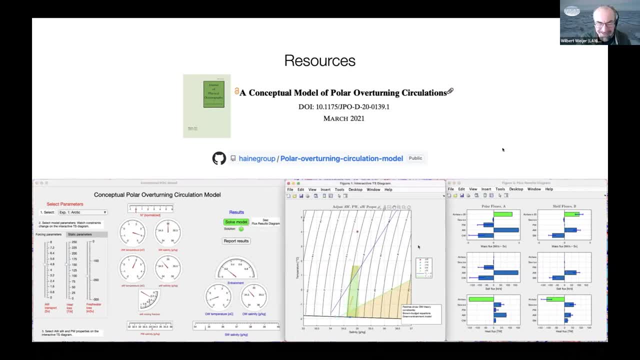 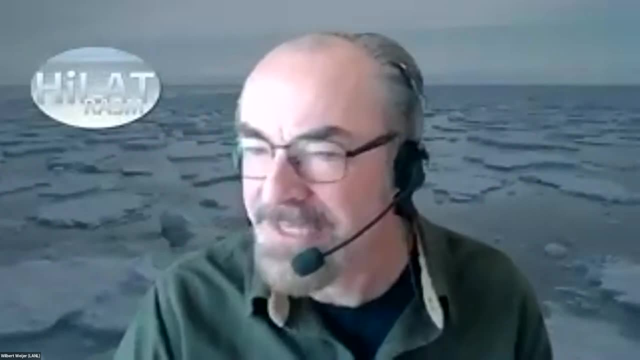 I mean, each of these presentations could easily have spanned two hours or something like that, And I'm really grateful for you guys to provide these very complimentary perspectives and very- yeah, from a really different observational and theoretical perspective. I understand that we have a little bit more time to go over the top of the hour. 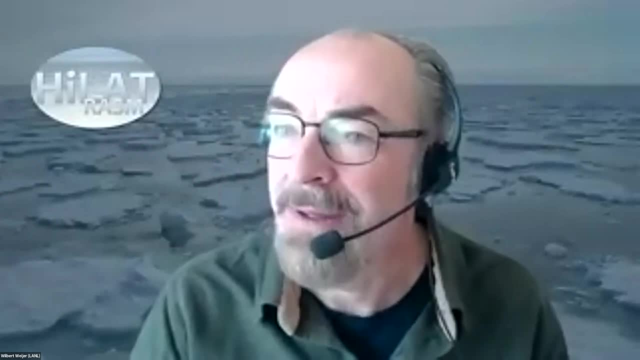 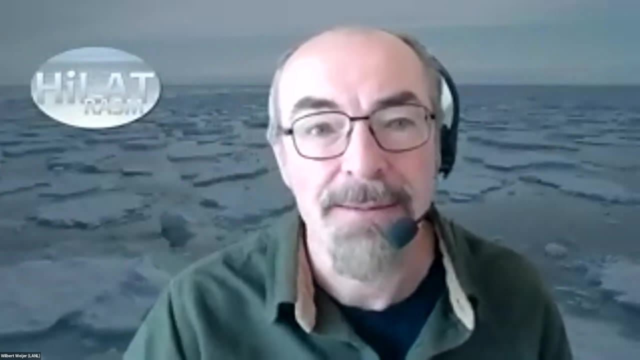 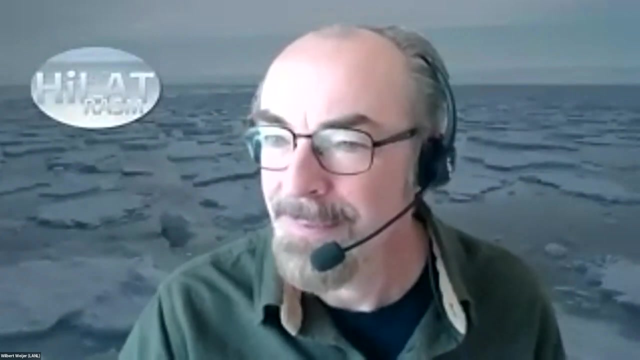 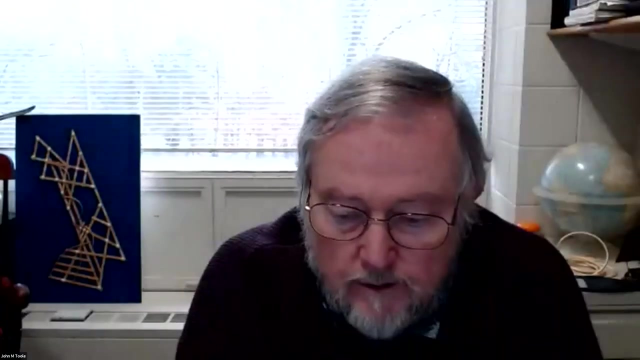 Okay, I do realize that many people may have to drop off at the top of the hour, So let's open this up for discussion. If you have a question, please raise your hand and we'll start with John John Thule. Thanks to both of you guys. 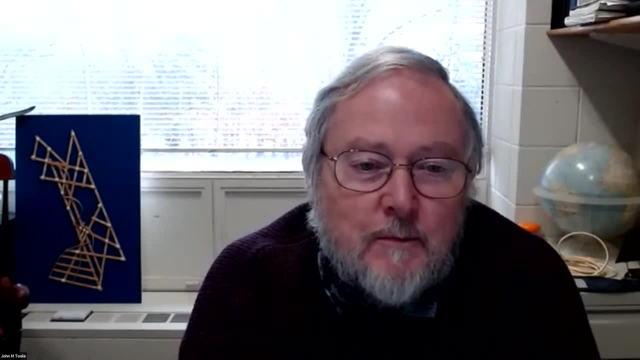 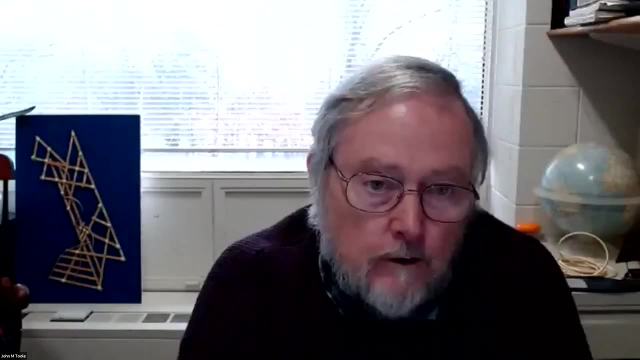 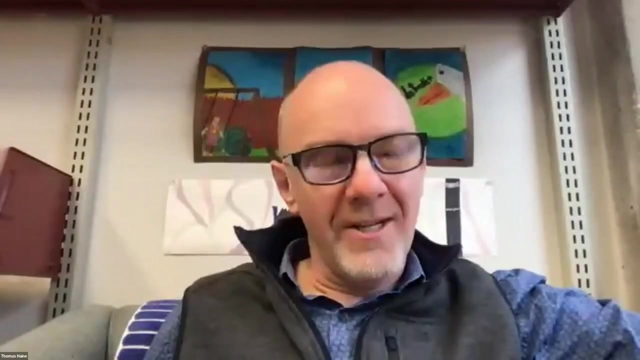 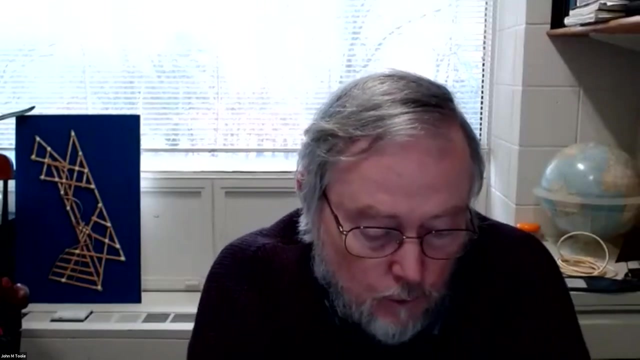 Tom, I would say that was very Rudel-esque presentation. You said nothing about the flow of the Pacific water into the Arctic and out. You just add that as a pass-through in this scheme. Essentially, yes, Yes. So a master's student did a thesis with me recently. 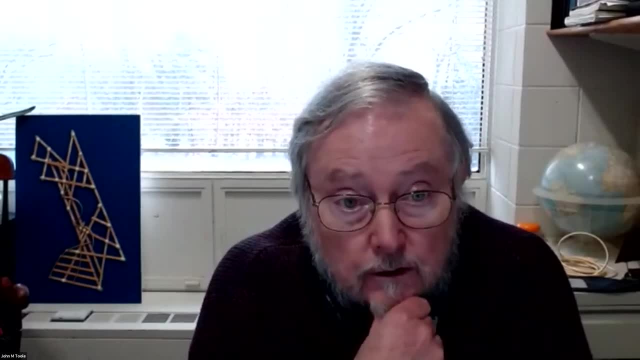 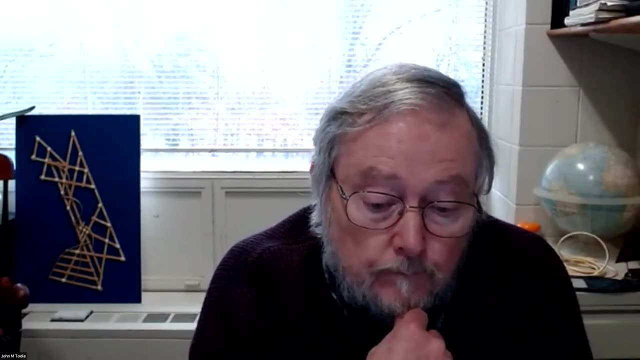 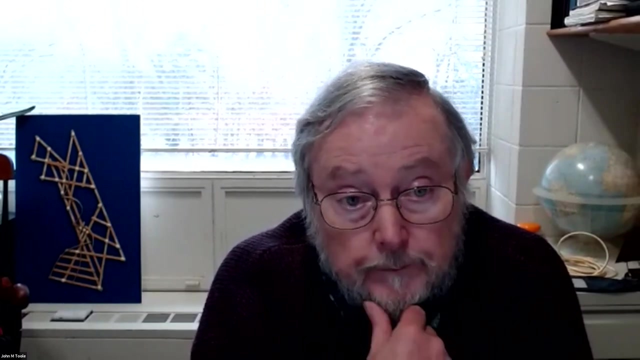 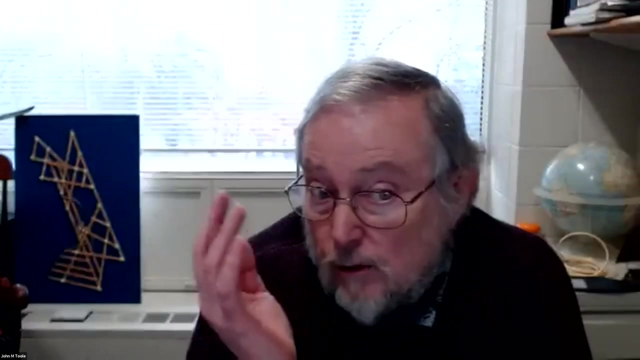 where we looked at basically the same three layers as you have in on-winds ASTA simulation And we actually got a stronger conversion of Atlantic water to polar water than bottom water. But that's a medium resolution model And I don't know what the exchange mechanisms. 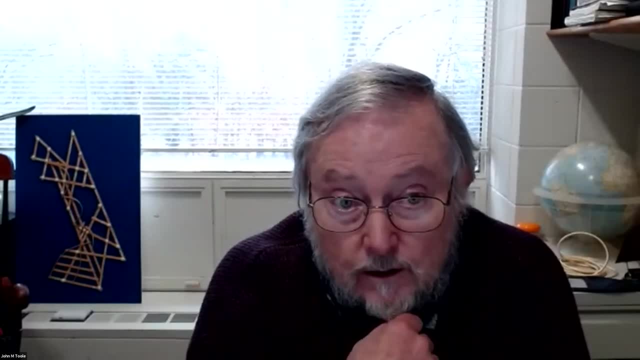 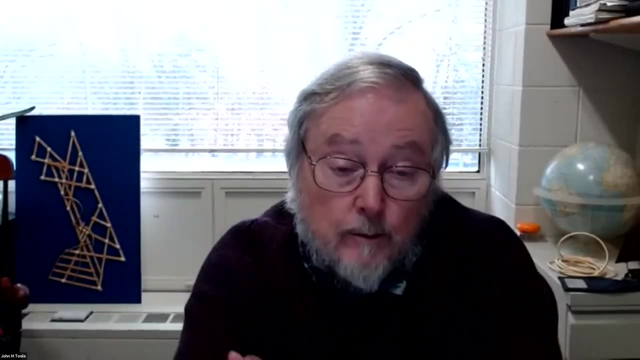 in the model being the shelf and the deep ocean are, And I think that's critical. Those transformations and entrainment are critical- And a model that has 10 kilometer resolution. I don't know how those are represented, So very interesting. 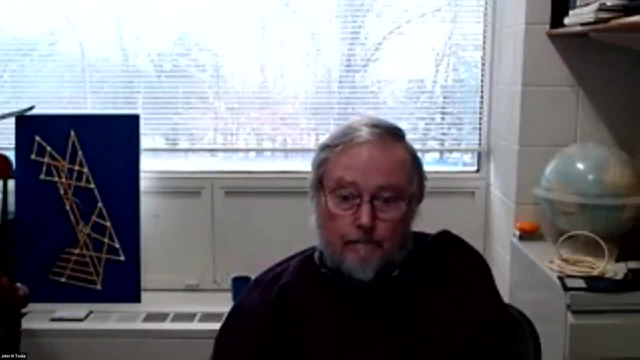 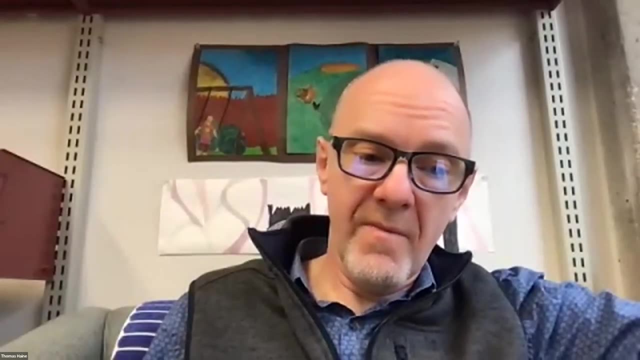 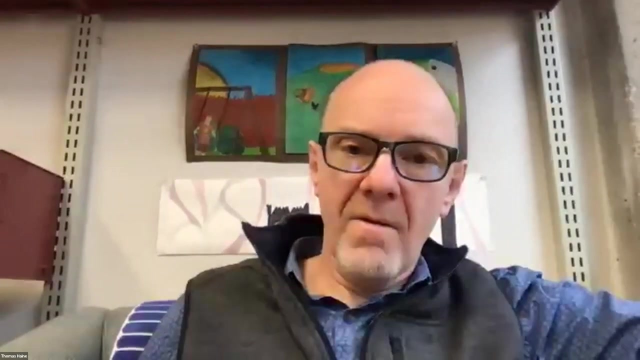 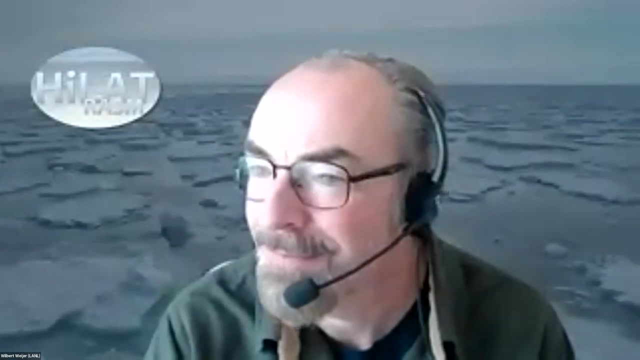 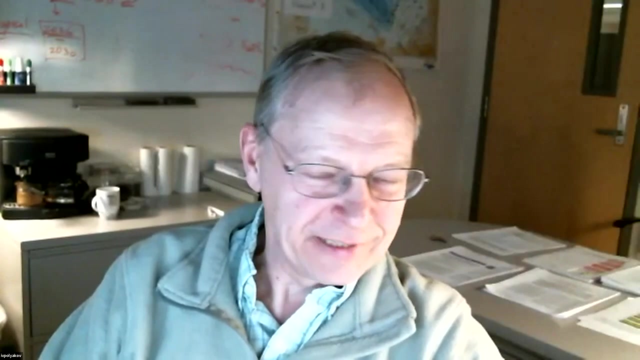 Thanks, I think poorly is the answer. I mean, the overflow process, of course, is at really small scales and high frequencies. All right, Dimitri, do you wanna ask your question to Igor? Yeah, trying to answer by writing, but i can answer without writing. 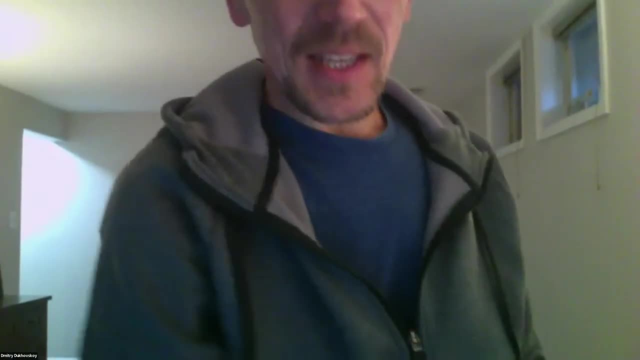 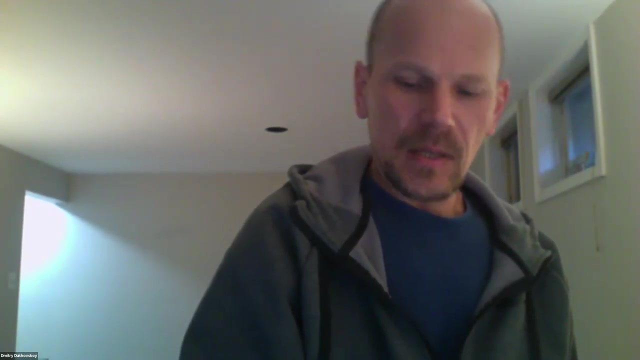 yeah, yeah, i'm trying to turn my camera on. i have several displays. yeah, yeah, thank you. thank you both for the presentations. it's, it was really interesting. um, eager, uh, my question is, um, about the negative feedback mechanism that could result from this increased ice melt. i wonder if this can. 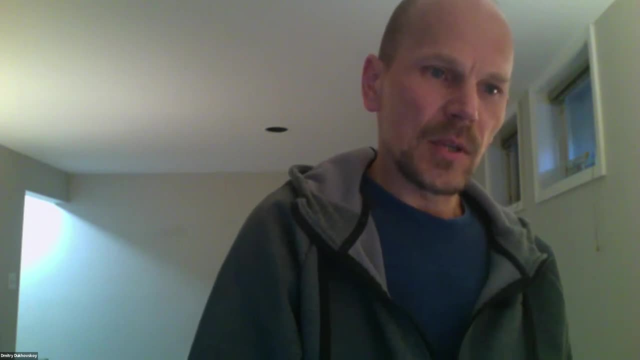 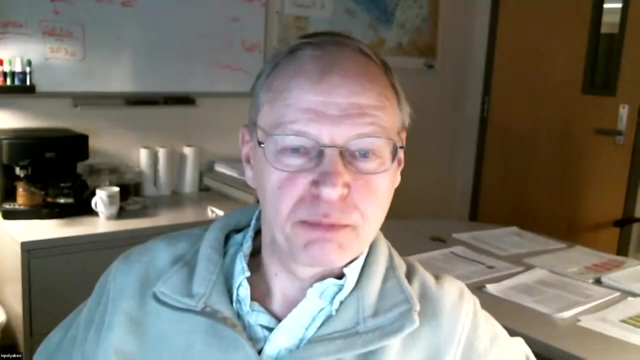 reduce the vertical heat flux that you talked in your presentation and return the system to the pre-authentification state. any comment about this? any thoughts about this, how possible it is? thank you, basically my um presentation, i hope, showed that this process of atlantic water heat ventilation occurs in. 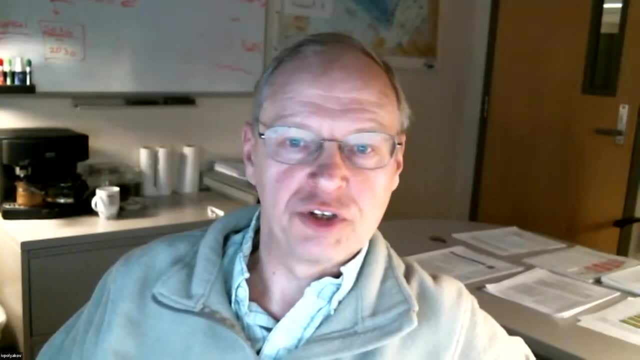 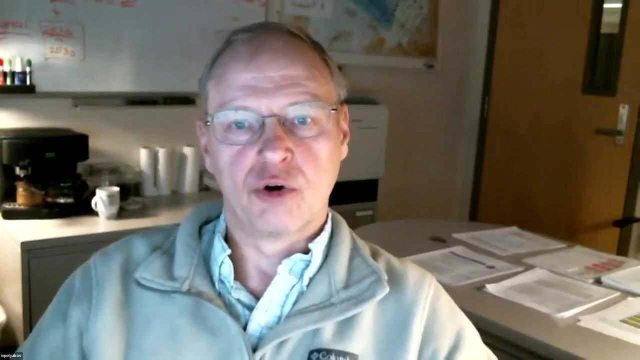 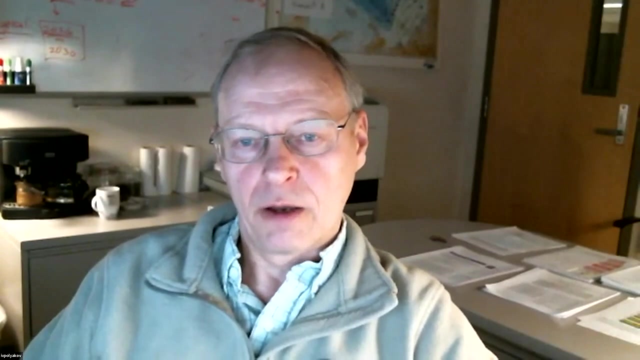 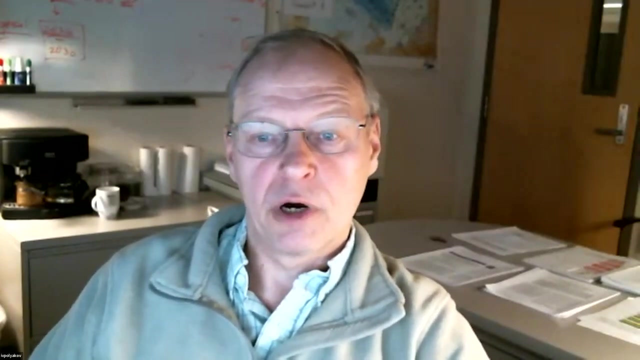 winter. this is a winter process with ventilation associated with cis formation. so both weaker stratification induced by advection of denser water from the balance c plus enhanced cis formation lead to ventilation of the upper ocean and that impacts cis formation. so this is not about cis melt, because 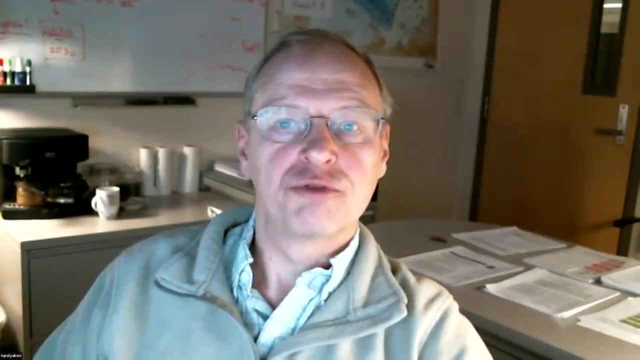 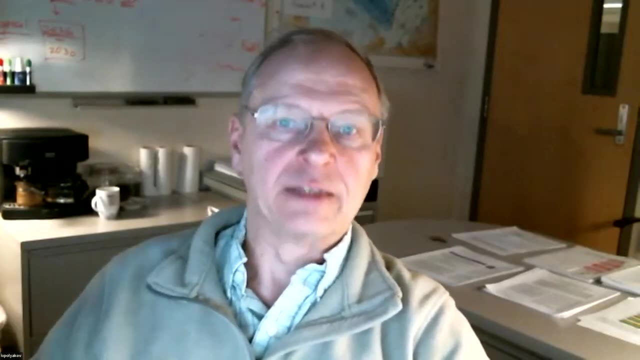 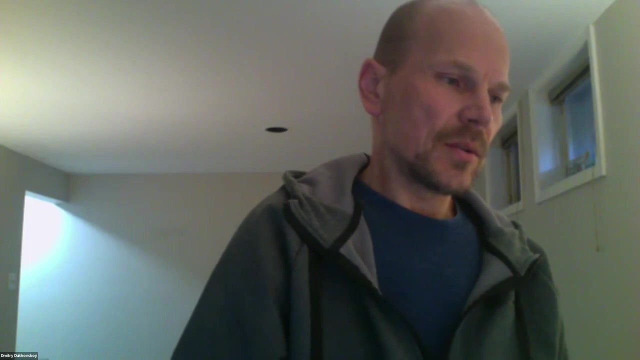 this is a winter process. this is about decreasing of rate of cis formation in winter so that preconditions ice for summer melt. so it doesn't create fresh water, it creates less. so i understand this, but in general, the increased cis melt would result in a higher fresh water content, right? so it will. it will precondition. it will precondition lower heat flux in winter, but overall there is less ice now in eurasian basin than before. so if you even melt all ice and then freeze the same amount, that would result in basically balance. but what i'm saying is that in winter there is less ice formation. 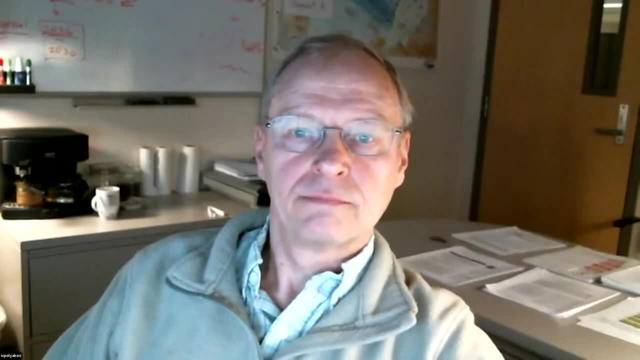 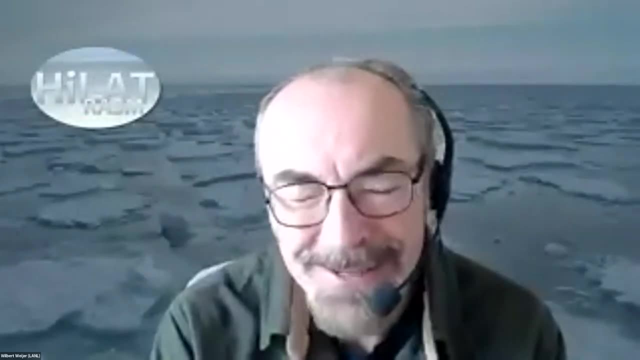 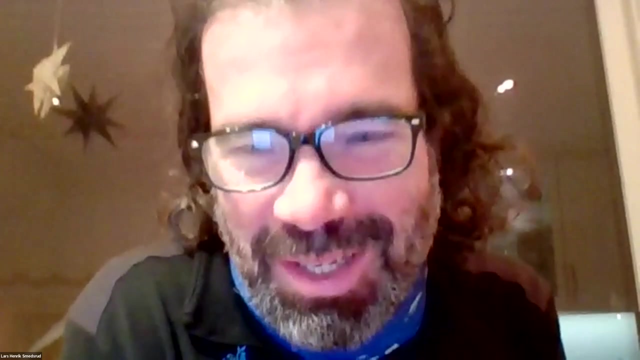 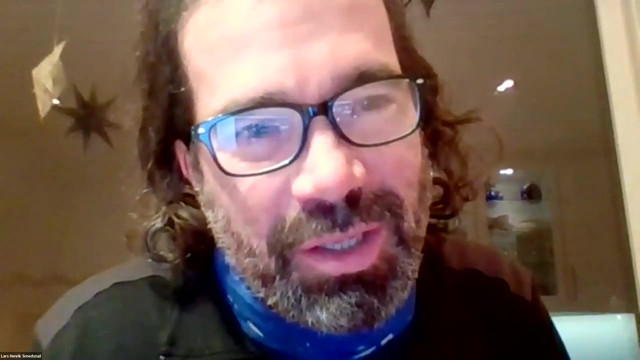 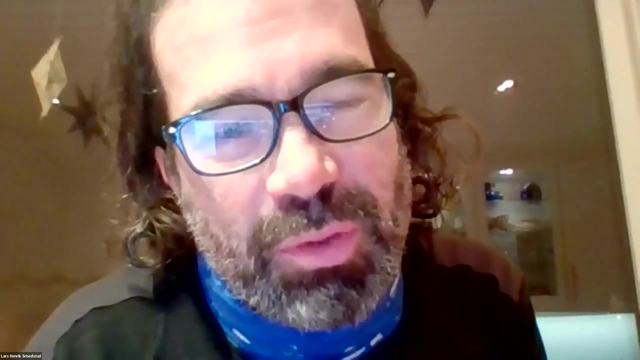 okay, thank you. any more questions for igor or tom lars, hello, yeah, maybe a simple question for tom at the end here. so i mean one of the most simple things that goes on. i think you know we are losing the arctic sea ice. this creates a larger portion of open water and this increases the heat flux to the atmosphere. 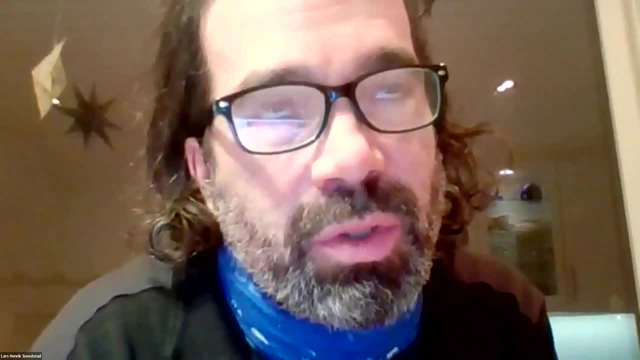 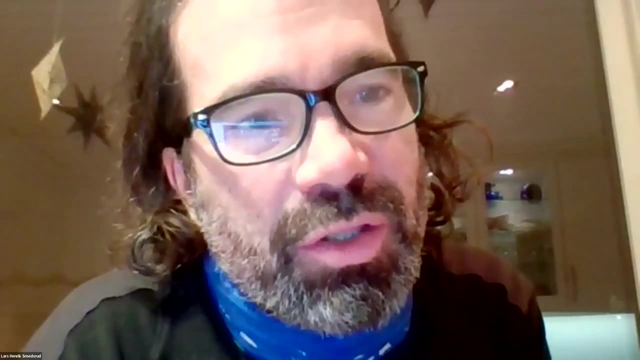 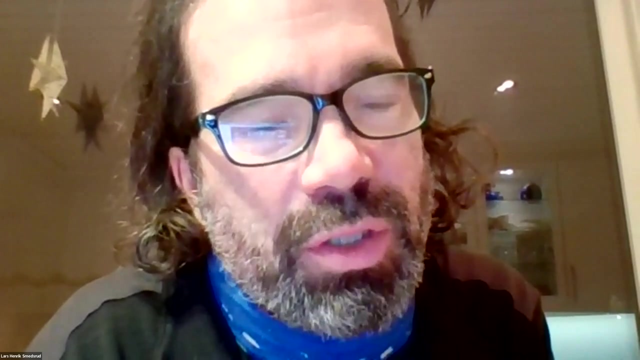 at least in the areas where we're losing that sea ice. so so to me, i think you know, a big question is whether this increased heat loss is is driving a larger atlantic inflow, and and in i mean, couldn't your model answer that question? or i mean, somehow you keep the proportions of this polar water and 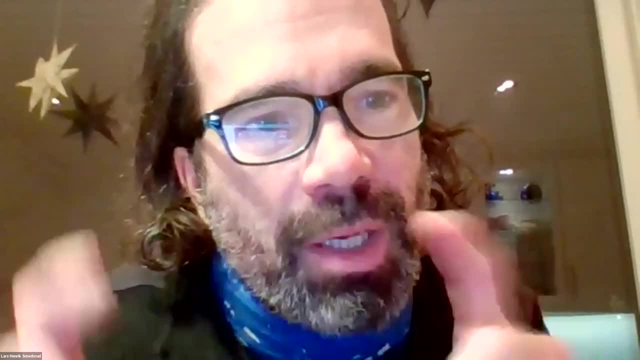 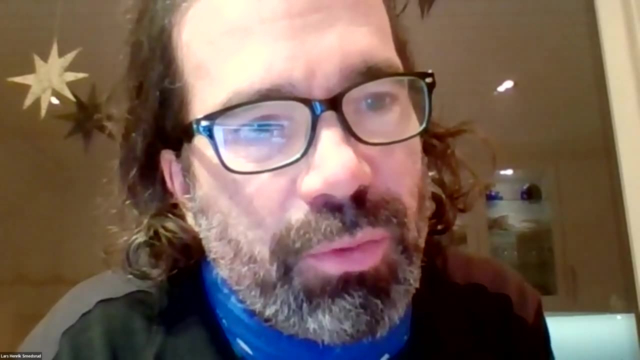 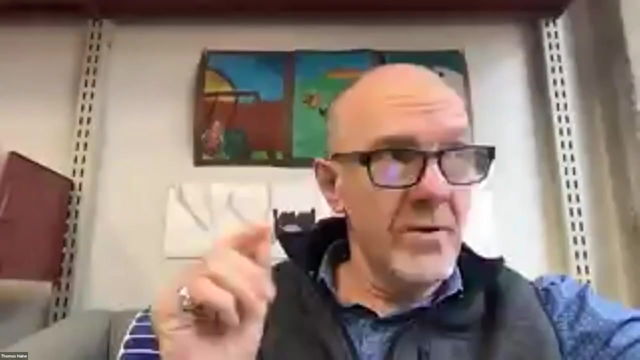 the overflow water constant. i mean they make so, but could you test a larger heat flux on the on the atlantic water inflow volume? um sure, so. so the relative amount of overflow water and polar water is not fixed. in the two examples i showed it happened to be the same, but in general. 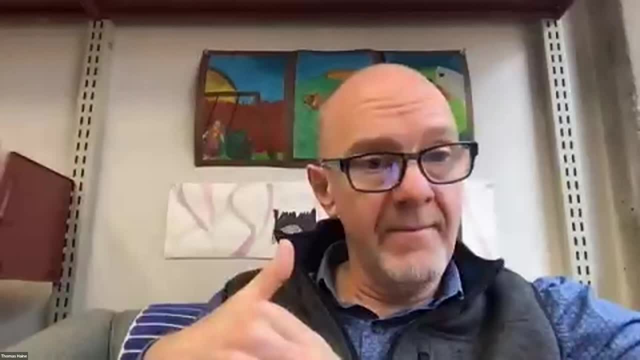 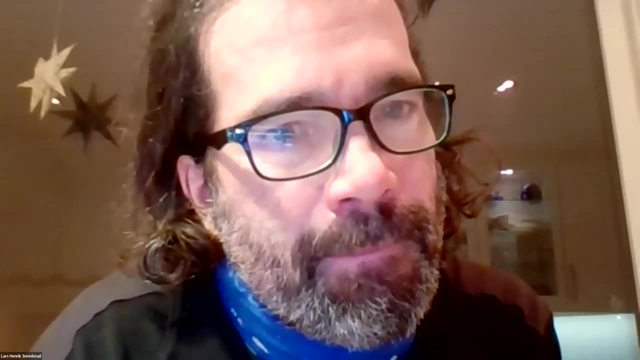 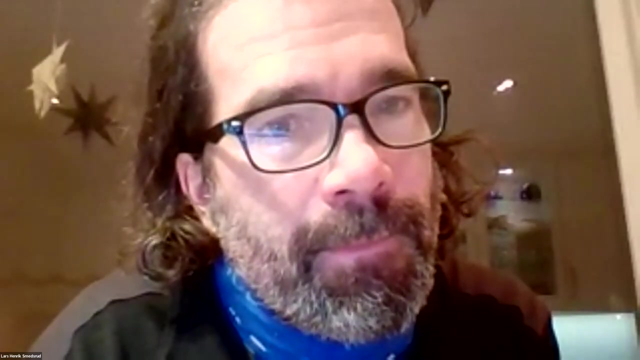 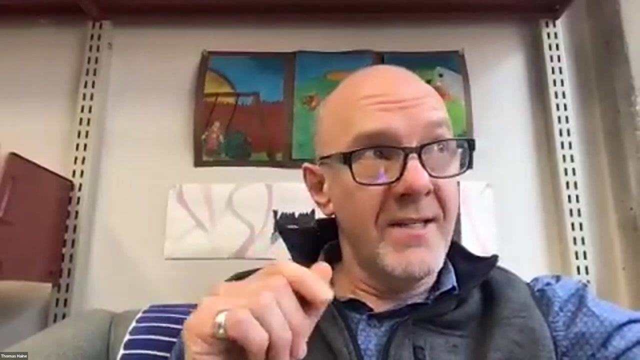 it can vary. so the atlantic water can be converted entirely into polar water or entirely into overflow water that emerges from the model, and sure you can vary the atlantic water volume flux, the atlantic water heat flux, as you wish. the heat crisis that i mentioned means loss of polar water, so that 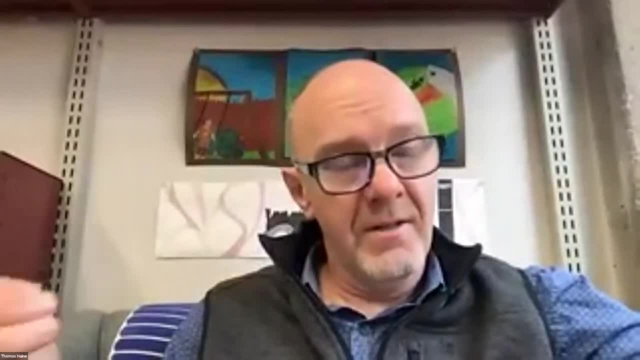 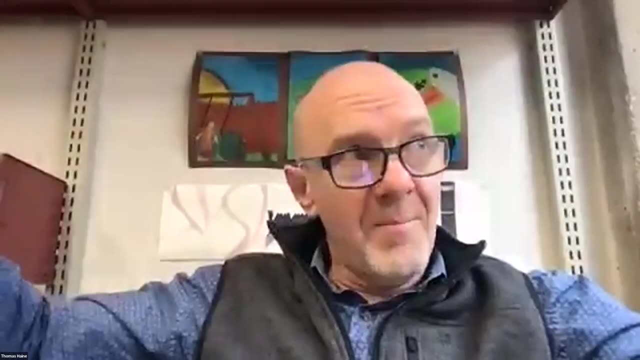 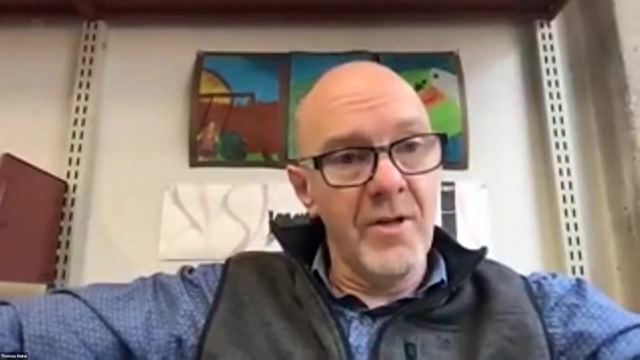 at least in the context of this simple model, is atlantification, so you you no longer have sea ice and um the beta ocean. then what tends to happen, of course, is that you get um thermal convection so you lose heat to the atmosphere, but the water is above the freezing point and it 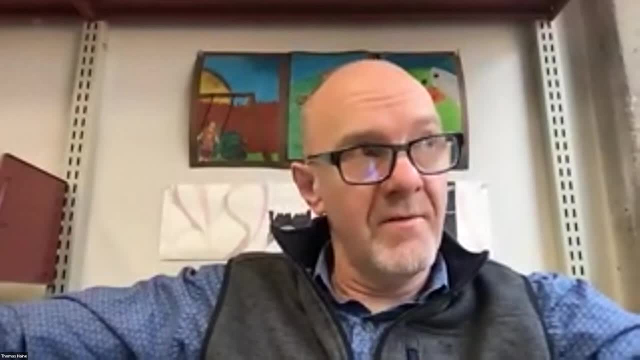 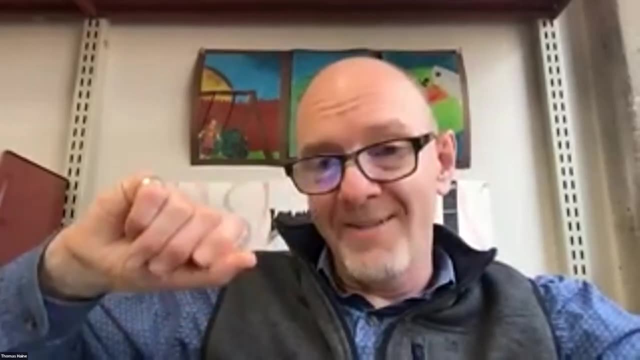 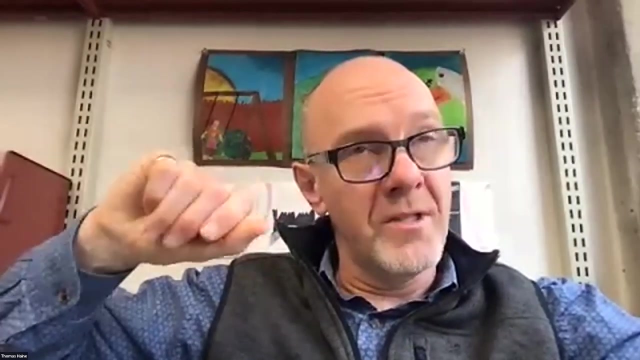 convects to great depth, like it does in the labrador sea. that process is not in the model that i just described and i would love to include it, but i don't really know how to yet, because i don't know what determines the fraction of atlantic water. 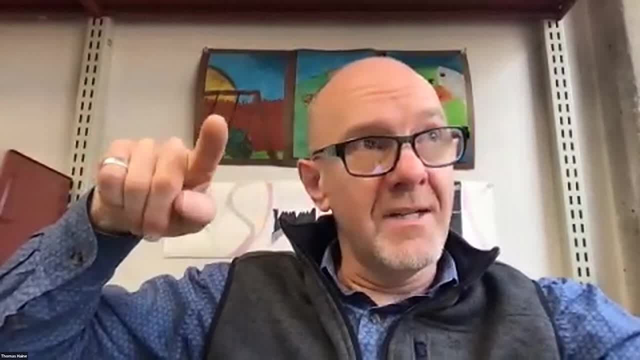 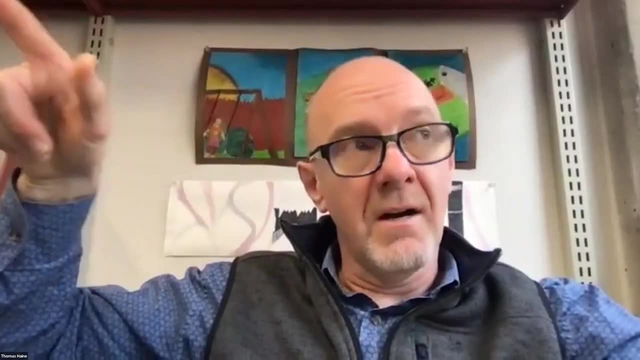 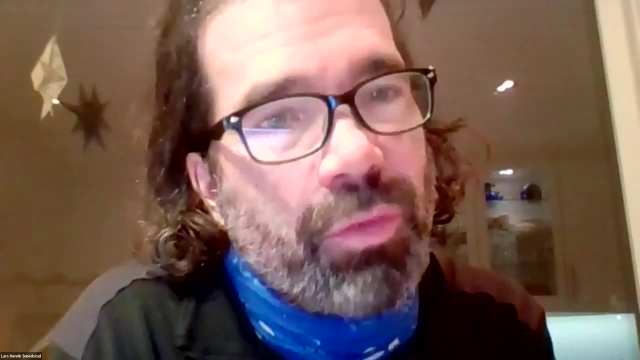 that is converted to overflow water via that deep convection pathway, versus the fraction of atlantic water that goes into the arctic and does this shelf interaction or sea ice interaction that i talked about? okay, i don't. i i want that to emerge from the model. i don't want to specify that fraction. 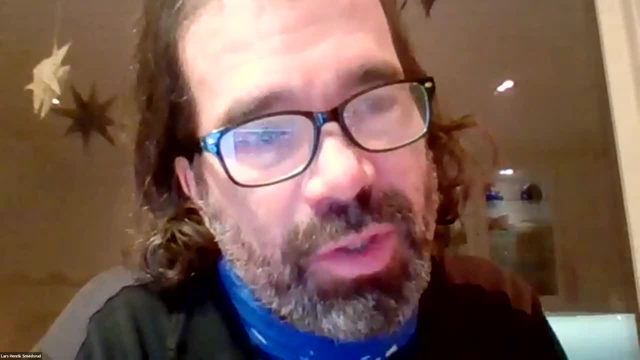 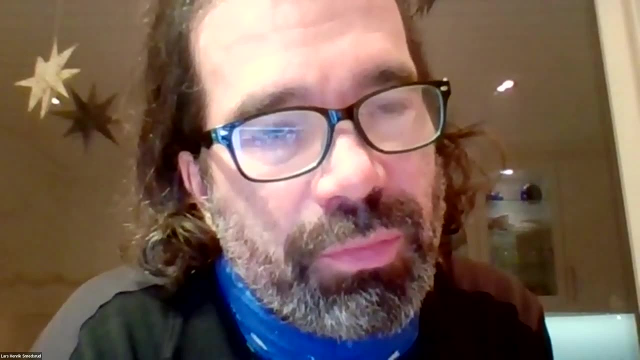 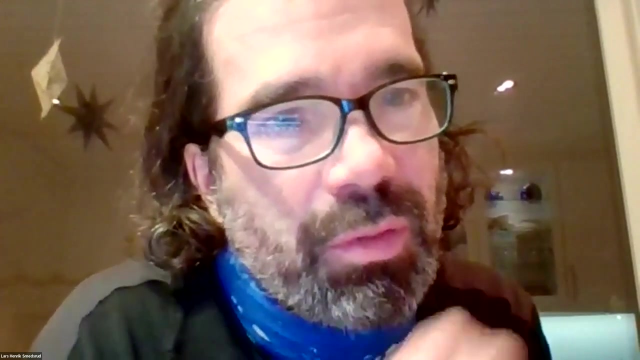 but that's just the cooling it's i mean. so what happens in the beren sea is that you have this atlantic inflow, it's largely just cooled and then it creates denser over. you know by that that simple cooling just creates dense water, which doesn't really change the salinity, it just cools it. so yes, 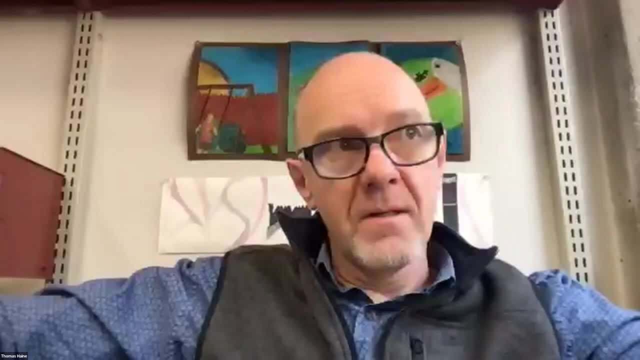 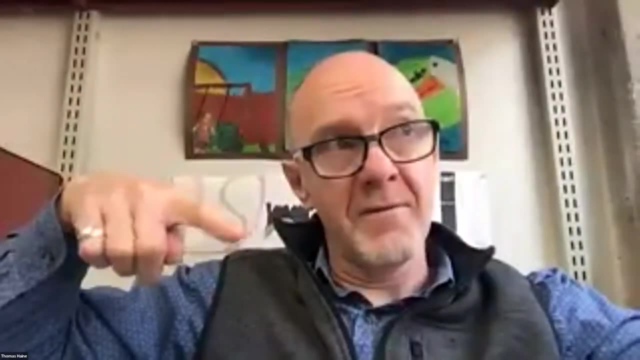 but so. but for example, if you think about what happens, the fate of the water which flows across the brilliant scotland ridge, like in the norwegian current part of it, goes, recirculates south into the greenland sea and then ultimately into the sub polar north atlantic. 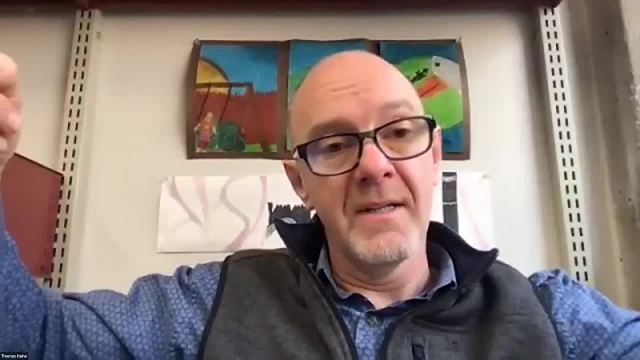 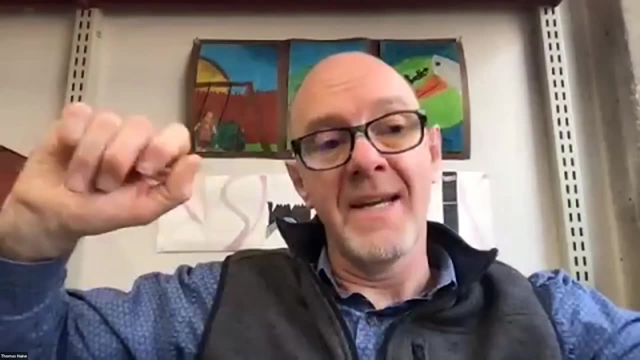 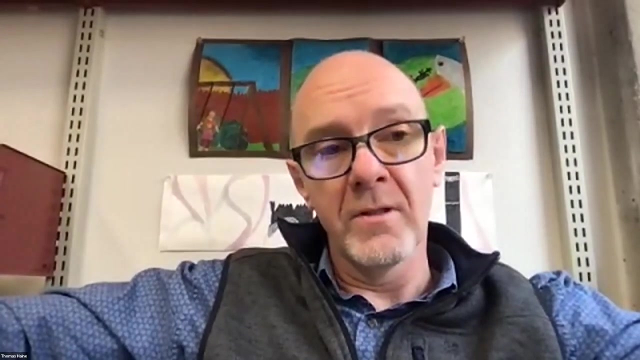 and undergoes thermal convection. part of it goes into the arctic and doesn't- or at least historically it didn't- very much. i don't know what determines that split, okay. what fraction goes back south? what fraction carries on north? okay, yeah, i mean, i would love to hear ideas if you have. 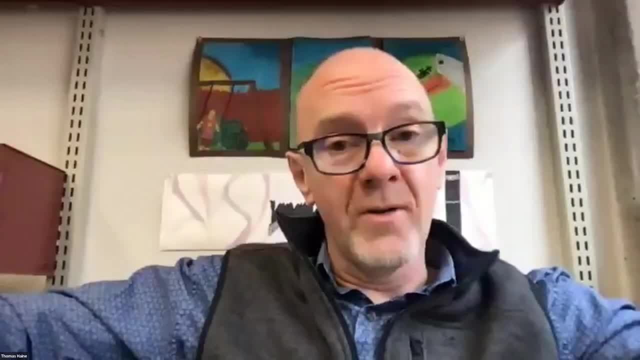 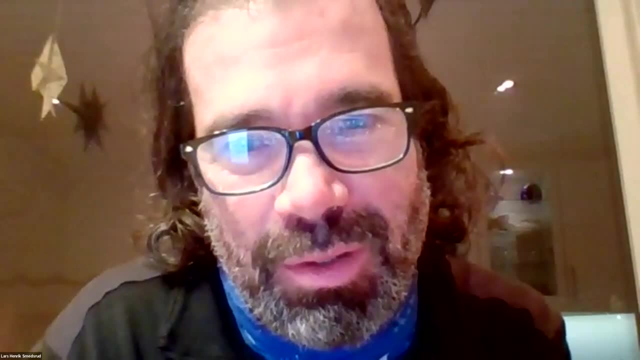 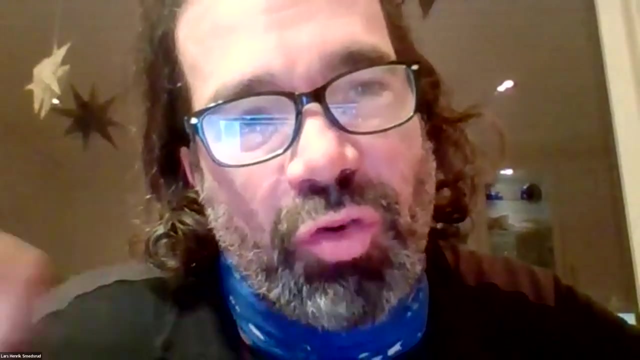 ideas about how to specify that. i'll think about it, and i i mean, if there's time, and one same i mean very, also very nice presentation by igor, but you know, but the main cause of what you see up there, which is very convincing, is that just a stronger atlantic inflow. then would that explain. 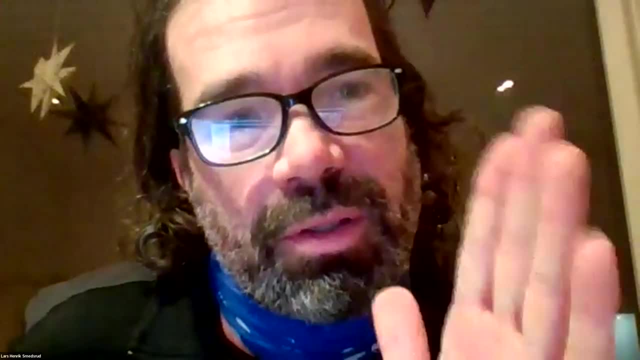 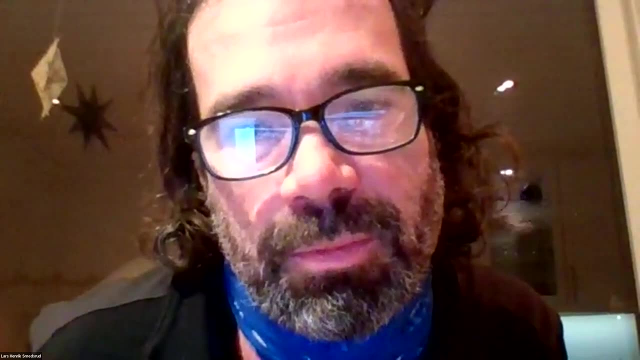 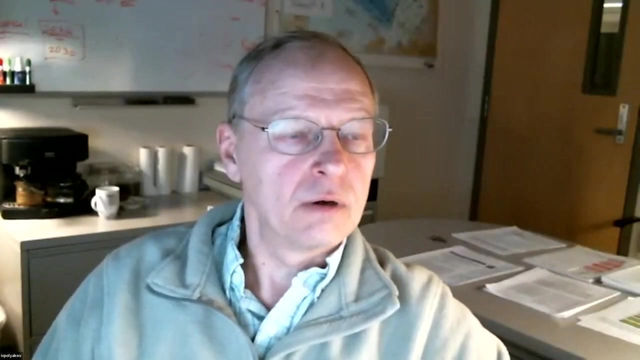 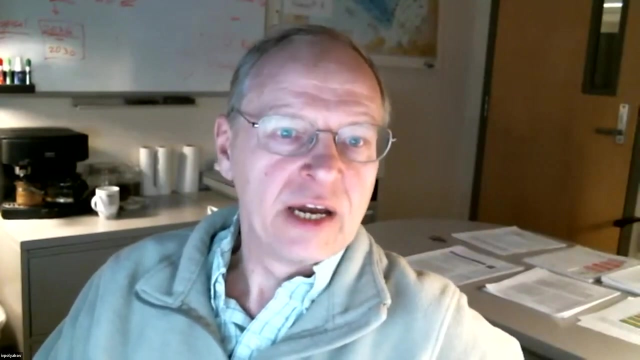 so this, so this deep, this steepening of the salinity at depth igori, that's just that- could be explained by just more atlantic water, couldn't it? that's what you're saying? yeah, our recent analysis definitely shows that this signal, this stress strengthening, this weakening of the arctic halocline is due to advection of what denser waters from the northern. 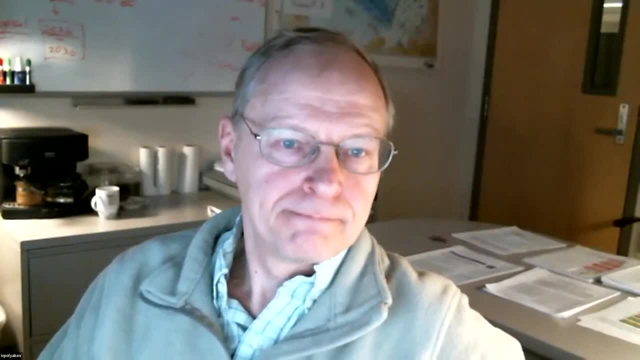 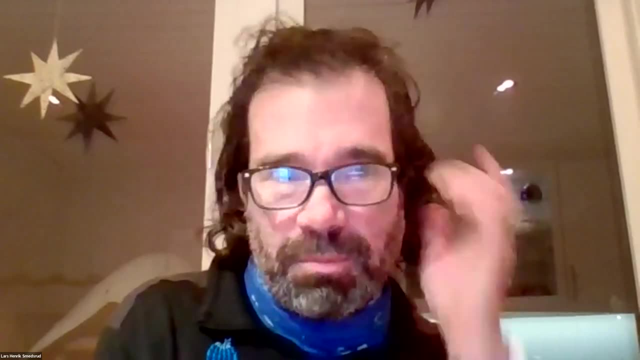 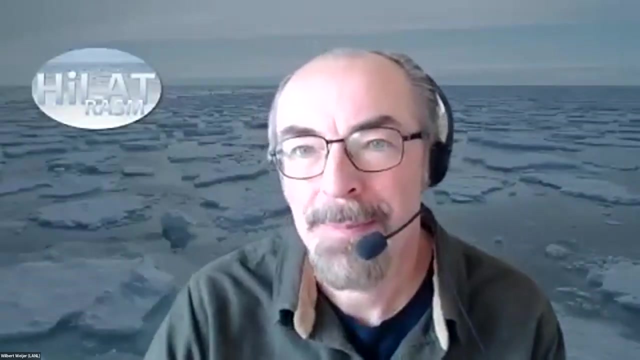 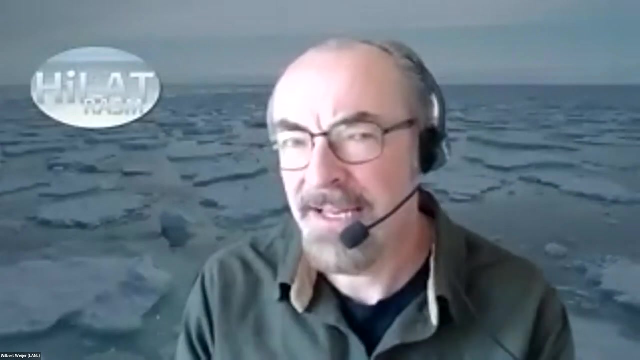 barren sea. okay, thank you. very close to you, very interesting. any other questions maybe? just for me to follow up on last question to igor: um, so is it then clear then what causes that enhanced inflow? is that a kind of a greater push from the, from the south northward, or is there also maybe a 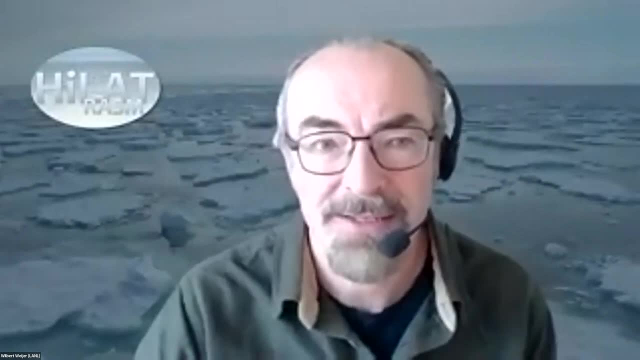 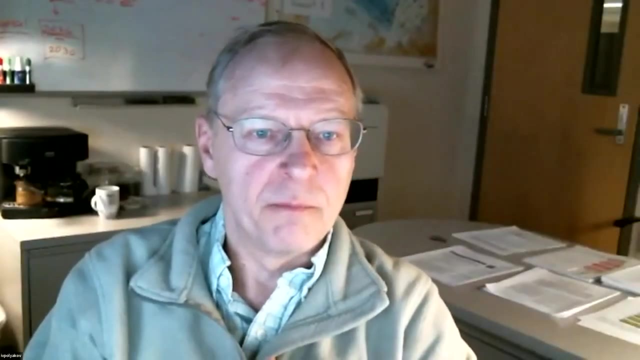 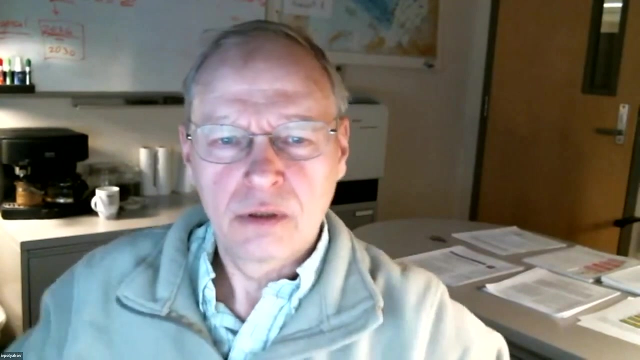 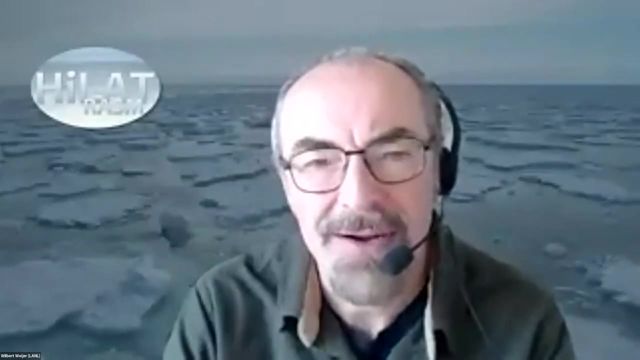 and a pool component that could be maybe consistent with some of the stuff that that tom presented. are you asking about this? differences in the barnes sea opening inflow versus from straight in floor? um, in general, i suppose the the enhanced inflow of atlantic water into the arctic. i think the strong role plays the atmospheric. 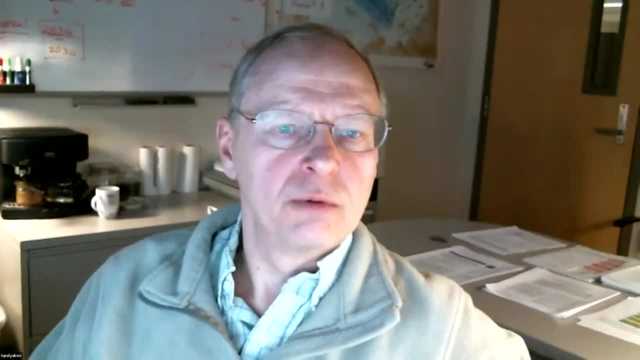 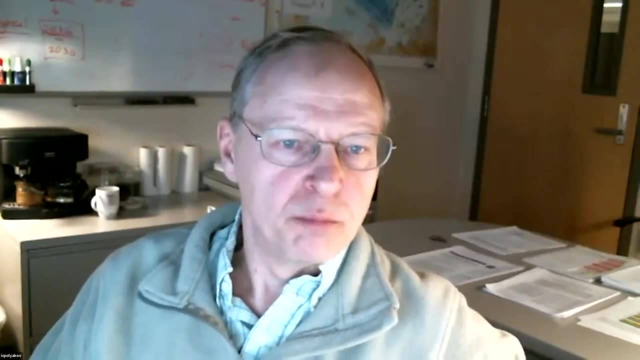 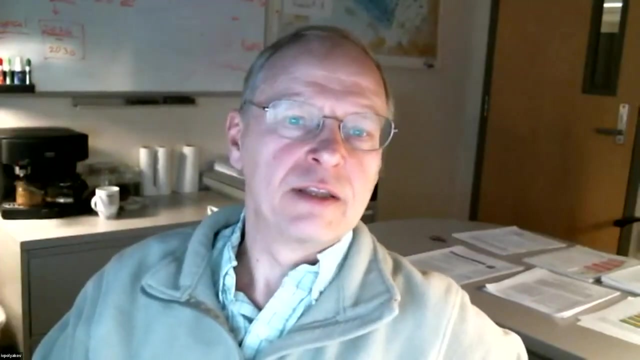 cyclonicity, anti-cyclonicity. that's what we are currently doing- this analysis- and we definitely see that the current atmospheric regime pushes more water through the barren sea, as i showed in my one of the first slides, then through the fram street, and that makes very 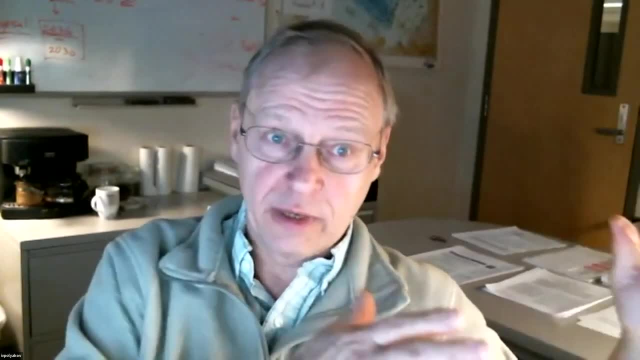 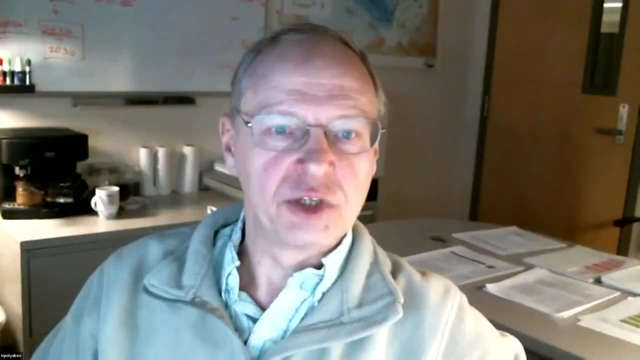 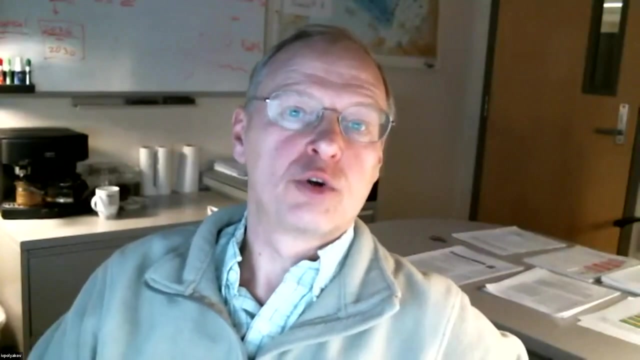 important changes in the arctic, so i was showing that atlantic water after 2007- 8 became a little bit cooler. this is very consistent with more uh important role of barnes sea water entering the arctic ocean than from street and there are many other uh evidences like like, like that. so 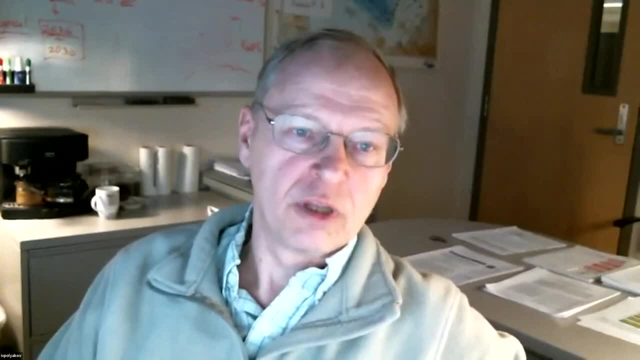 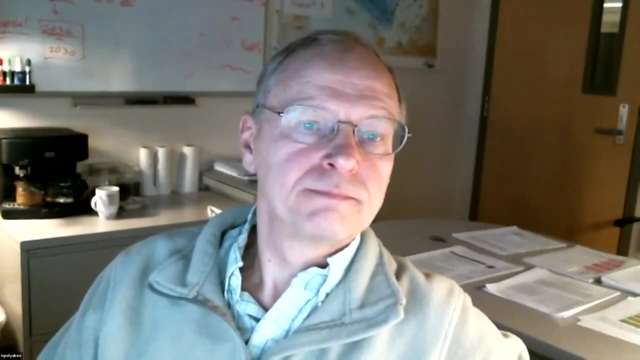 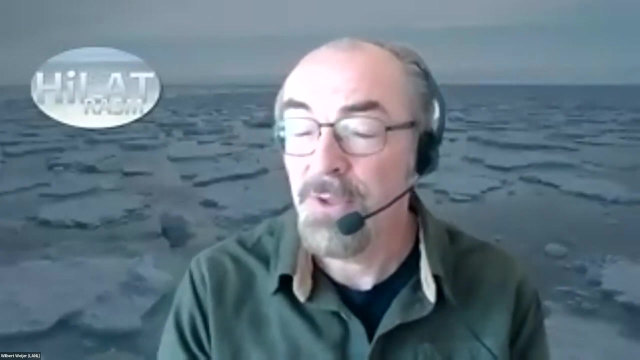 definitely, atmospheric circulation plays a very important role in shaping, uh, the influx of atlantic water into the arctic ocean. and is the distinction, then, between the inflow through the fram straight or the barnes opening? is that, then, just due to the different ways that the ocean then interacts with the atmosphere?